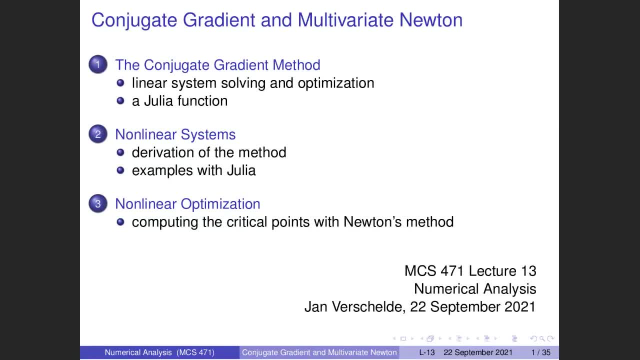 And they're the Jacobian method Positive definite matrices. And these matrices occur when one applies Newton's method to finding critical points of a vector, Or actually of critical points of a function in several variables. The Hessian is actually the Jacobian of the gradient vector. 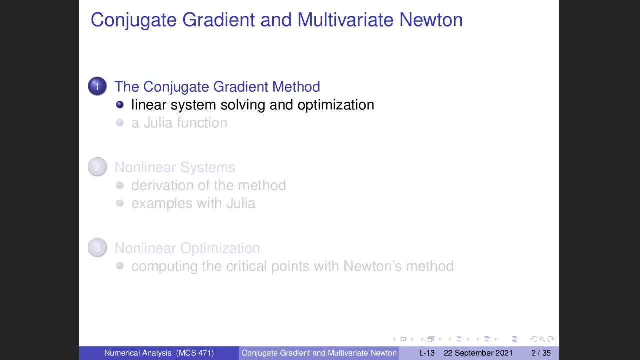 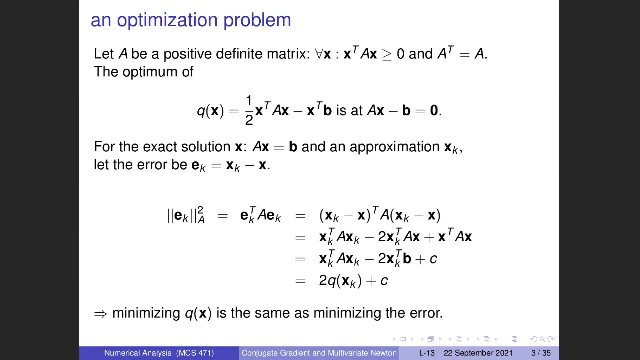 Alright, so let's dive in. So we will see how linear system solving connects with optimization. So in the last lecture we've seen how a positive definite matrix Actually here it's still a positive semi-definite, If you allow equal signs here. 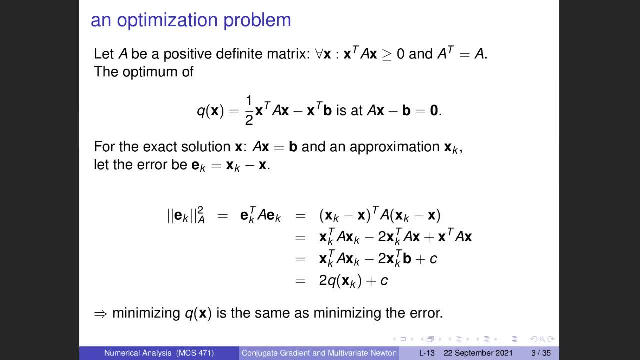 But in short, every matrix leads to a quadratic form if it is symmetric and positive definite. So the symmetry is that when you transpose you get the same matrix back. Now let's look at a very particular quadratic form. It's given here by this Q. 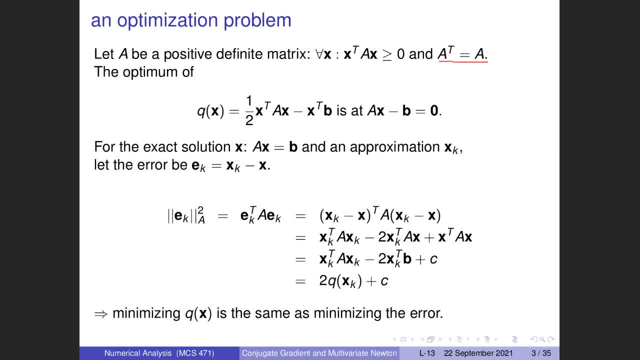 Now, if you take, If you look at the gradient, If you look at the vector of all the partial derivatives, Where Q of X equals zero. This is when you have that AX minus B equals zero. So now we have a quadratic form. 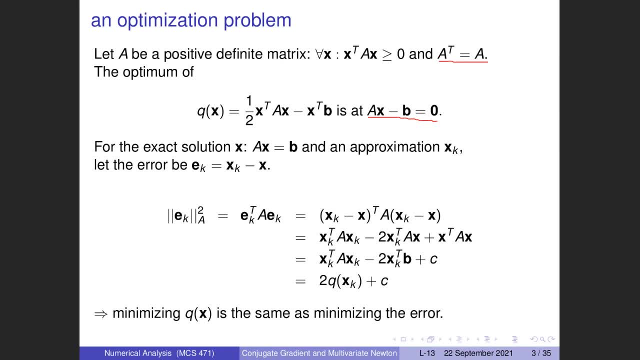 Specific quadratic form defined by a matrix and the right hand side vector. The connection between optimization And the solving of the linear system is that if you compute the optimum of the quadratic form, Then actually you are solving the linear system. So one could interpret this as an application of linear system solving in the way I just explained it. 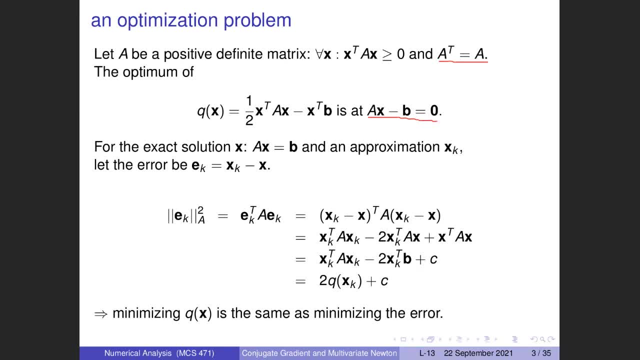 You take the derivative of the quadratic form and you get a linear system. So any quadratic system, quadratic form, will actually lead to a linear system. So we will not do that. instead, we will use ideas of optimization to get to a method for solving a linear system. 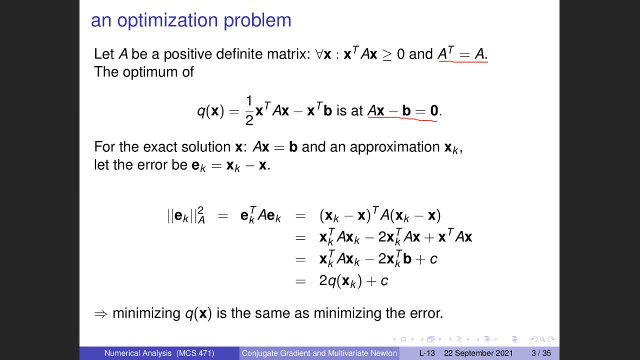 So we will introduce. So here is another way of seeing this: If we introduce a linear system, If we introduce a different norm- So we have the norm that has a subscript, the matrix- Then this is defined as this. So if the A is the identity matrix, 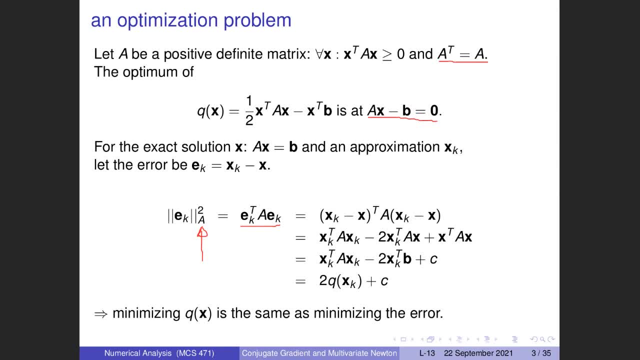 Then we actually get to the square of the Euclidean norm. So why do we do this complication? Well, look what happens. What happens is that When you write it out in great generality, We see that we return. We get the quadratic form back where we started, to it. 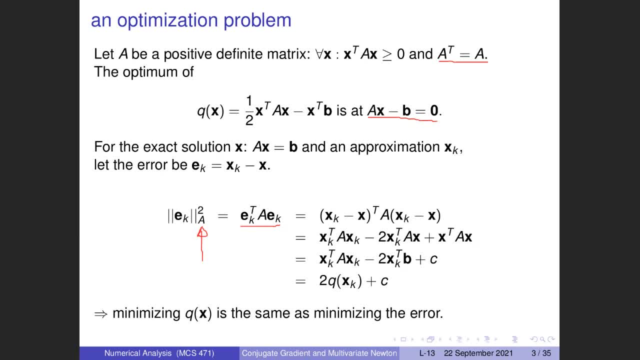 So our special quadratic form Q is actually equal to our norm, Our A norm, Our norm, Our vector norm that uses the positive, semi definite matrix A. So another point of saying that if you want to minimize the quadratic form, And we're going to minimize this quadratic form, 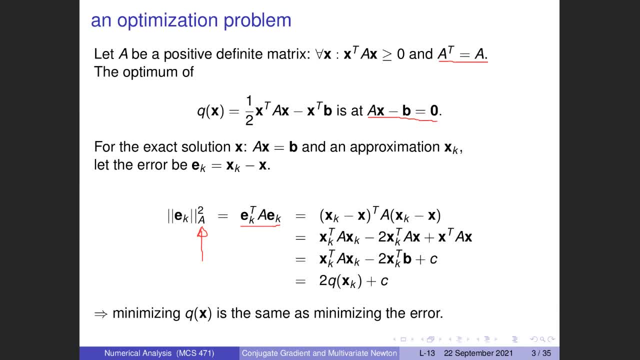 To solve the linear system: AX equals B. So if we can minimize the error term, Then actually we are minimizing the quadratic form. So one natural algorithm to minimize a general function Is to use the steepest gradient. So you compute the gradient at a point. 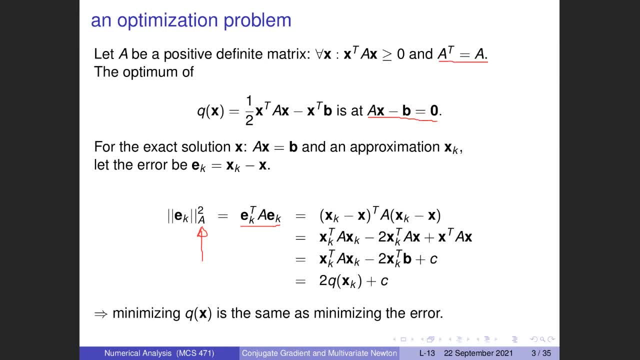 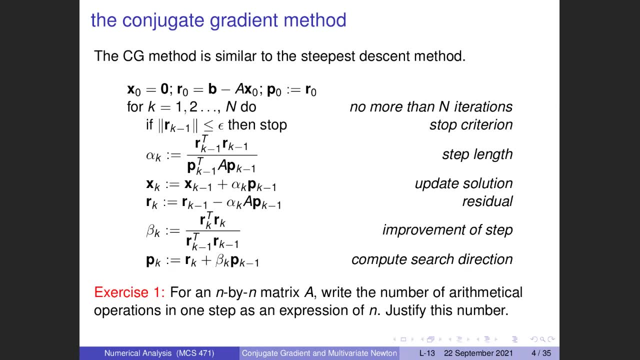 And then you go in the direction of that gradient. If you look for a minimum, You go for the steepest descent. So we will consider a method, An iterative method, That is fairly similar to the steepest descent. So the steepest descent is a very simple method. 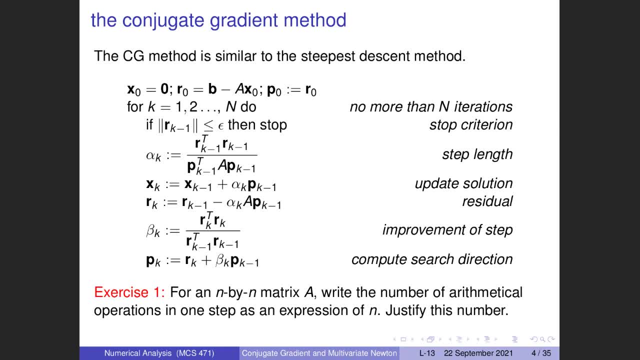 But we will make it better And that will lead to the conjugate gradient method. So we start out here with zero. In a way this is kind of the generic starting point, But in many practical applications We actually know already A good start for our solution. 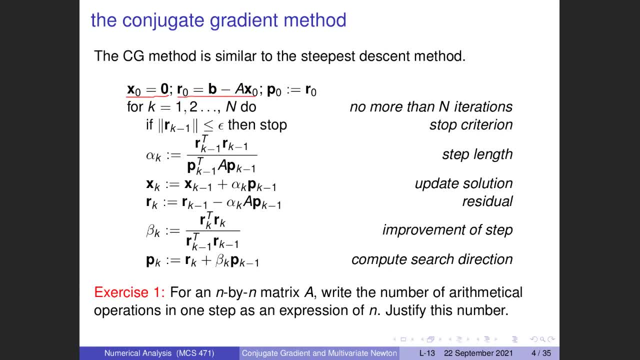 And we will compute the residual. So here you see that if the residual is smaller than our epsilon, We actually stop already. So the first stop criterion is taking the norm of the residual. So we will have a direction That is P, So we will walk into that direction. 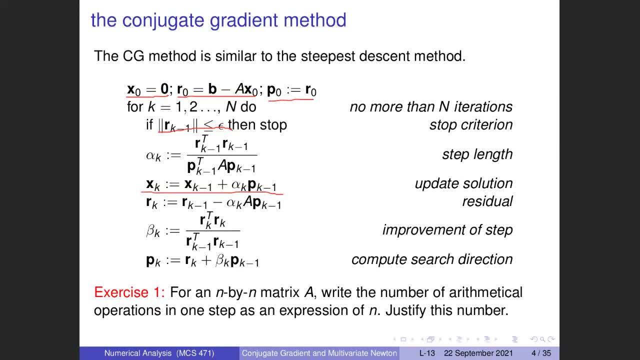 So here is the Resemblance with the conjugate gradient With the steepest descent. So we have a vector And we take a step in that direction. Then we update the residual And then we also update the search direction. 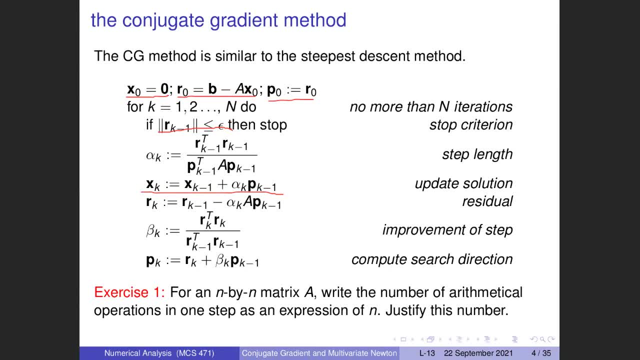 Now this algorithm depends on two critical quantities. So we have the step length, And then we have The improvement of the search direction. So we have an alpha and a beta, And in what follows I will try to explain The formulas. 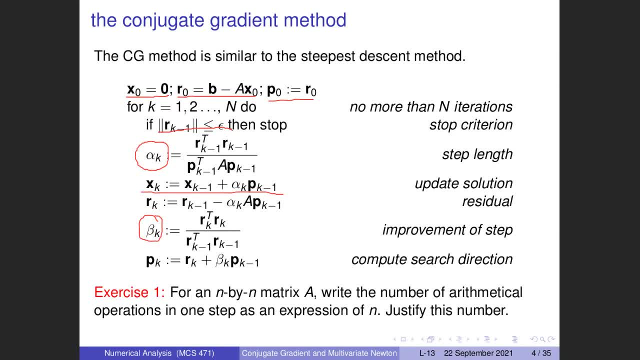 Why do we take The alpha and the betas Like the way we are doing? We have seen that last time That Koleski is actually twice as fast, At least twice as fast- as the LU factorization, But it is still a cubic method. 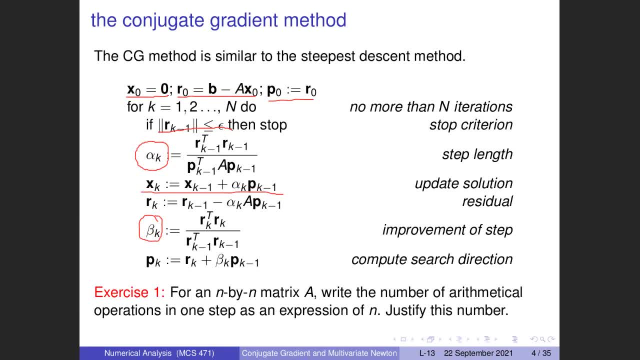 Here it is an iterative method, And iterative methods when they converge They have the promise of working with a quadratic cost. So the cost of the exercise. The goal of the exercise one Is to analyze The operations That are done in the execution of this algorithm. 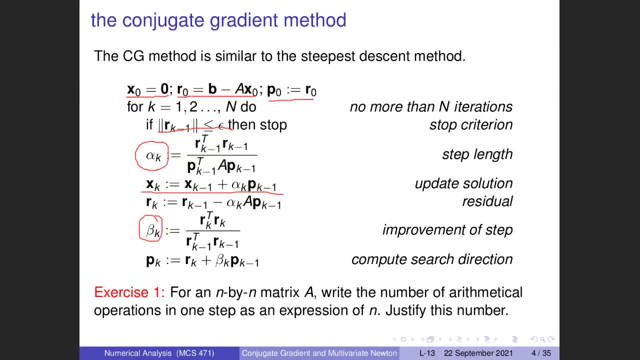 So one does a lot of, And doing this with the general For a general dimension. So you see that there are a number of multiplications. So here what I am underlining. now Perhaps I should have taken another color. I have A times the search direction. 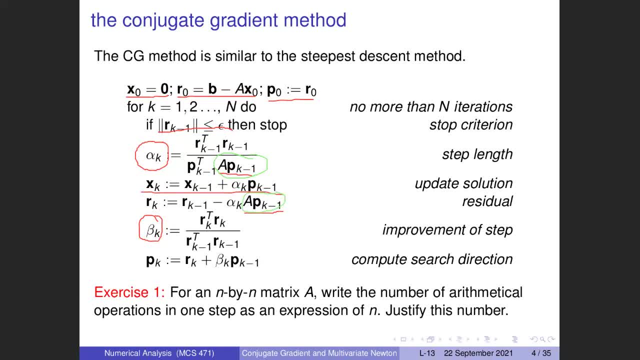 And the A times the search direction Comes back in. So we covered iterative methods before. What iterative methods are doing Is that they are doing matrix vector multiplications Repeatedly And I just circled in green The bottleneck. So my mathematical description. 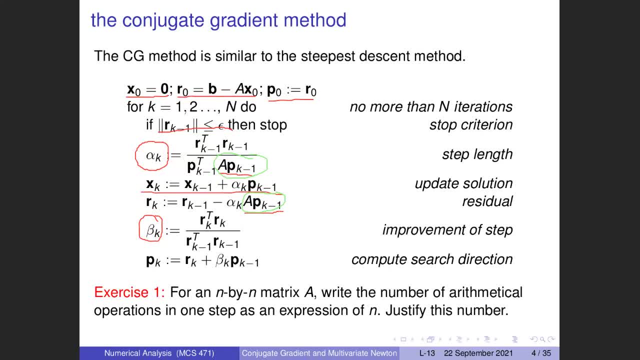 Does not use a separate variable For the A times P sub K minus one. But you could say that you do this only once. So in every step Here as it is written Now, we do two matrix vector applications. So the cost of every step is therefore: 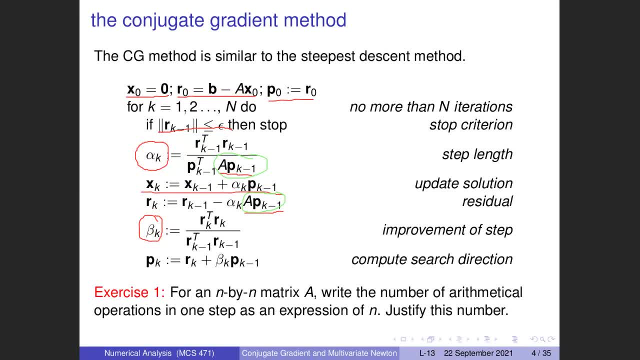 At least quadratic in the dimension, But if you look further. So what then remains So other than the green circled Computation? here, Either we, Either we multiply a vector with the scalar, Or we do the inner product Of two vectors. 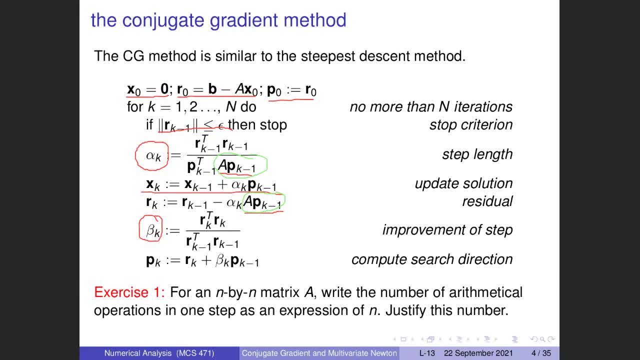 Or we do the product, So the inner product. If you store actually here the A Times P sub K minus one, What is here in the denominator Is again an inner product, And inner products are linear. So in solving this exercise, 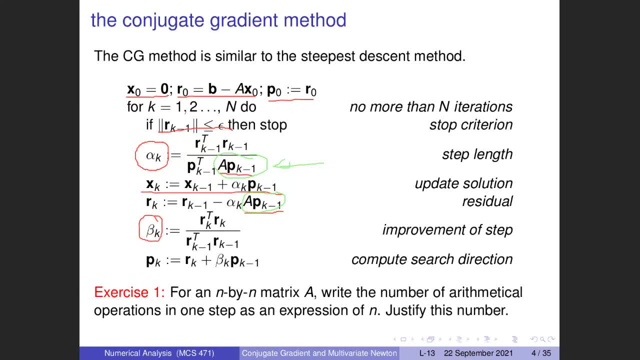 You point out that there are two Matrix vector multiplications And then there are a number of inner products And products with a scalar Which are both linear In the dimension. So the justification is important, So coming up with a neat expression, 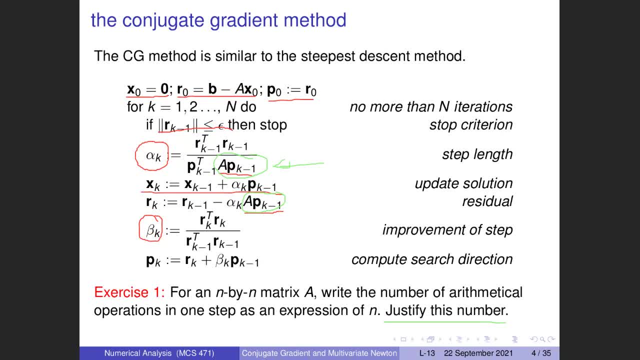 And we'll give you back some credit. So you can already write that at this Quadratic. So the one step means that You ignore the four. So it's actually what is Here in the body of the One step of 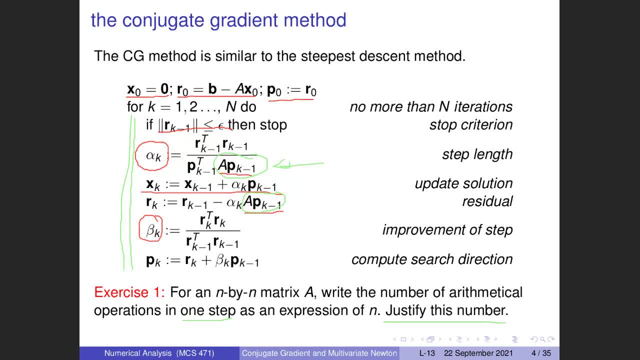 Executing The conjugate gradient. So this is the motivation. So we can Solve very large problems Still within a reasonable amount of time. So cubic algorithms Do not scale very well Once the dimension gets past Several thousands. All right. so 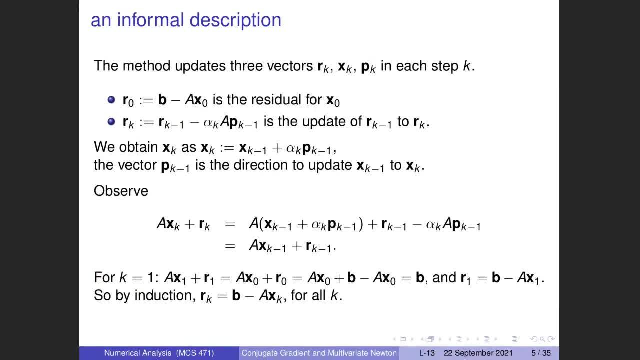 I tried to explain What the algorithm was doing, So here is a more informal Description. So we have three main vectors. We have the residual vector, The vector of the current approximation, The X sub K, And then we have the direction. 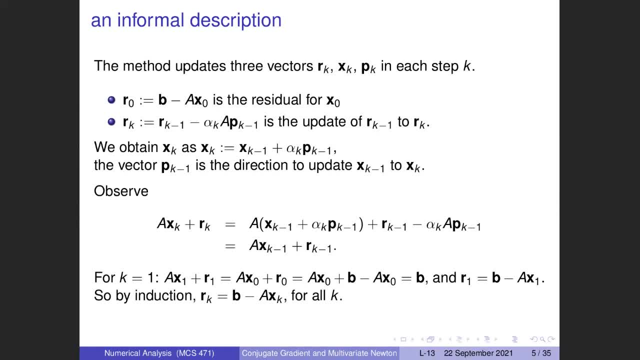 So these are our three main actors And they are changing. So the First vector is Perhaps easiest to understand. The first vector, the R, Is the residual, So this is also known as the backward error. How much should you change your problem? 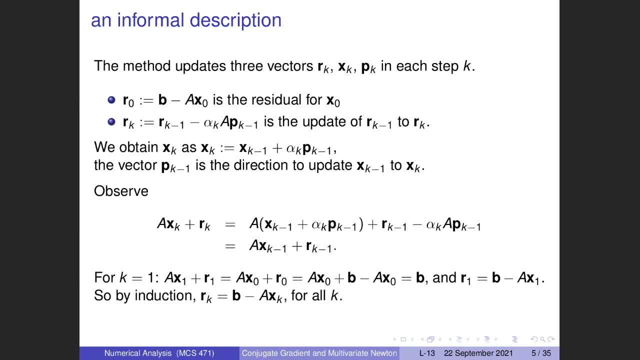 And in particular here the right hand side, Vector B. So the computed Vector is An exact solution. So the second actor Is then our Vector that we are updating. So here you see the update. Very similar steepest descent methods. 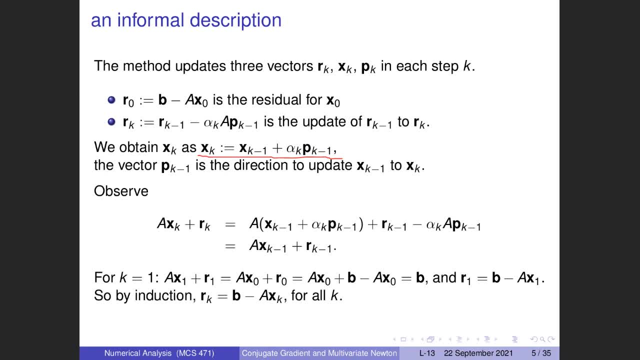 And then we have the vector In, which is the direction of the update. So these are the three Main vectors that are updated. We can already observe a relationship Between two consecutive R, K, R vectors. So the R naught is obviously the residual. 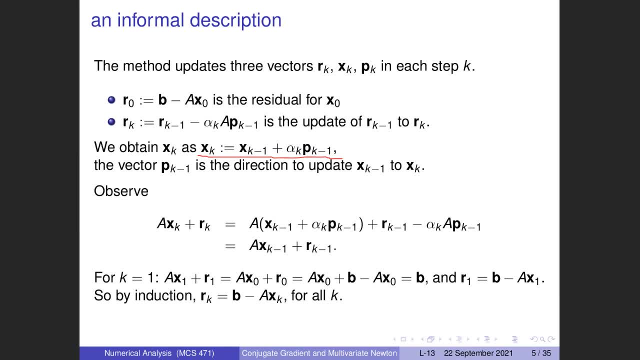 But it's not actually Obvious that the, That any other R vector, is also actually a residual, While this relationship actually Makes this clear If you substitute the definition of X K back in And then You Also Use the definition for the R sub K minus one. 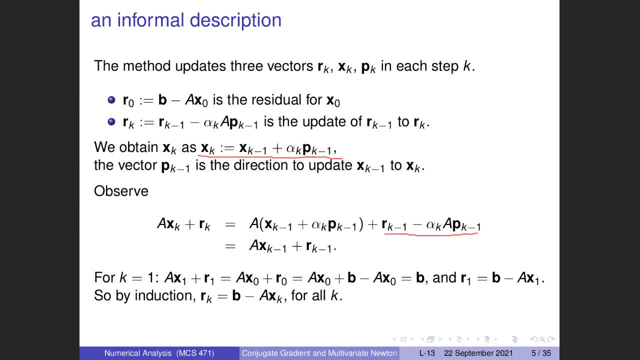 So the previous R vector. Then actually you see that there is a very neat relationship Between Two consecutive R Factors, And here This is made more explicit. So you can actually, Because of this relation, You can see that all the 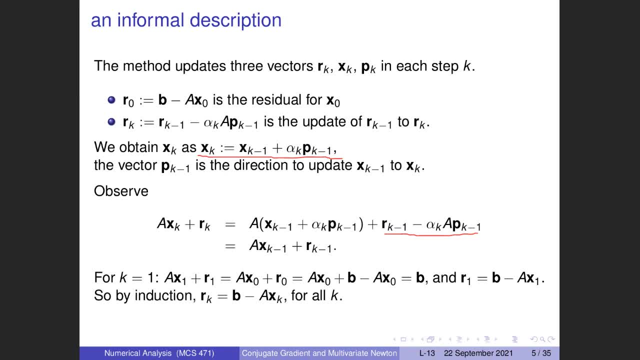 R vectors Are actually Relative To The Vector. R vectors are actually the residual Vectors. So the They measure the proximity Of the solution, The computed solution, to the exact solution. So that's our first Important 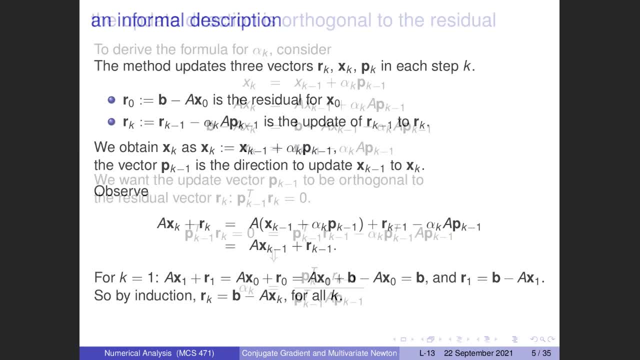 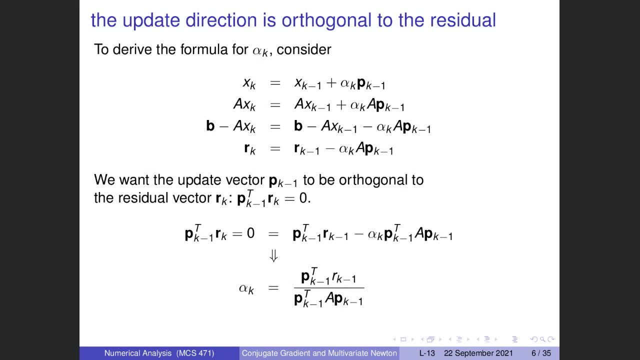 Relation On the Vector R. So let's Let's now look at Why. How do we choose the step size? How do We Update The Solution Vector, The approximation For the solution Vector? 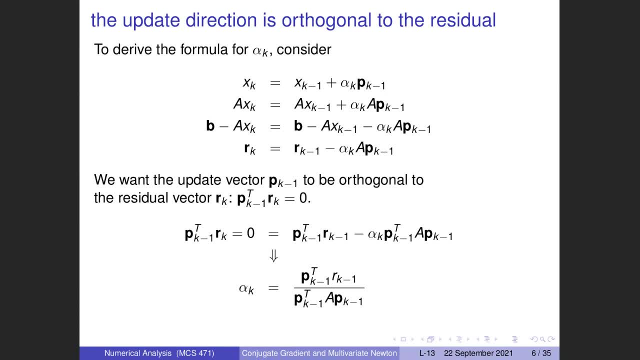 So let's Look at The Property Actually That We want. We want That The update Vector Is orthogonal To The residual Vector, So Orthogonality Will Play An important. 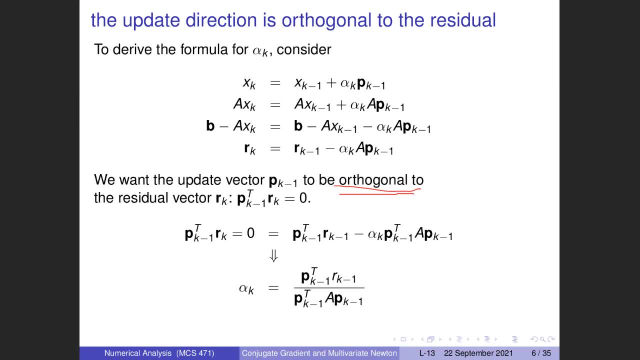 Role In this See. So Orthogonality Will Go Will Help Us A lot To Ensuring Orthogonality. So Here We Will Use The Orthogonality. 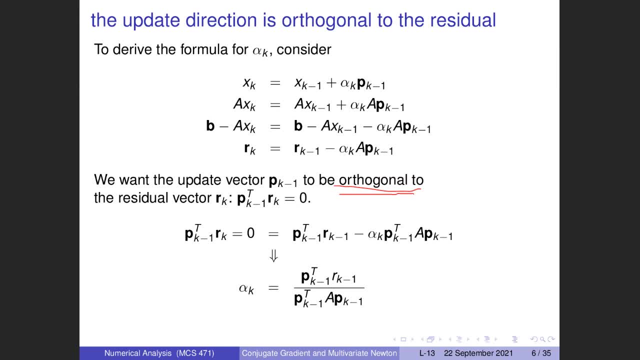 To Indicate That The Residual Vector And The Update Vector. So, By This Condition, On The Fact That The Update Vector Must Be Perpendicular, 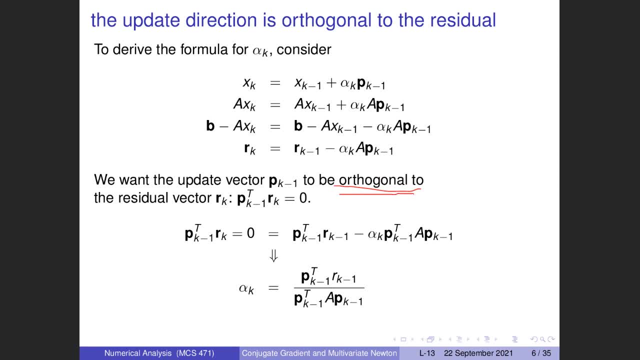 To The Residual Vector, We Obtain The Expression For The Alpha. So First We Do Rewriting, We See What Happens Here. We Actually Then 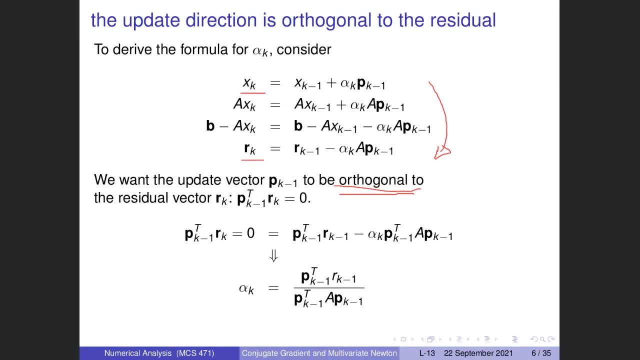 Get A Relationship Between Two Residuals, So We Want That The Arc Is Perpendicular To The Vector And This Will Lead To The Residual. 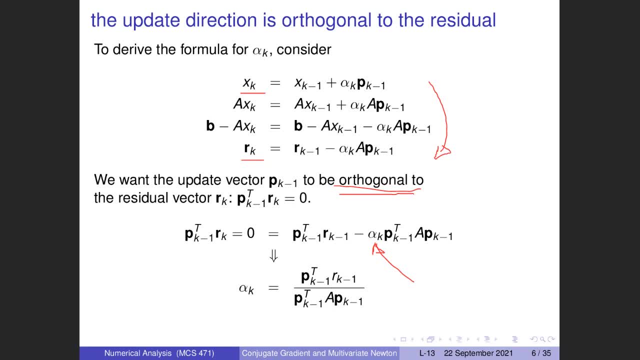 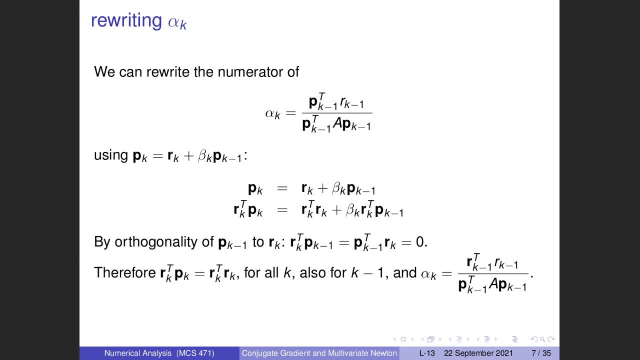 Of The Vector, So We Have The Residual Of The Vector, So We Have The Vector Of The Rectangular To The Vector, So We Have: 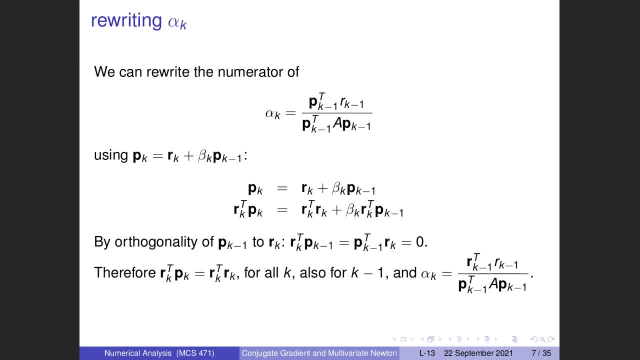 The Vector Of The Rectangular Of The Vector And We Have The Vector Of The Rectangular Of The Rectangular Of The Vector Of The. 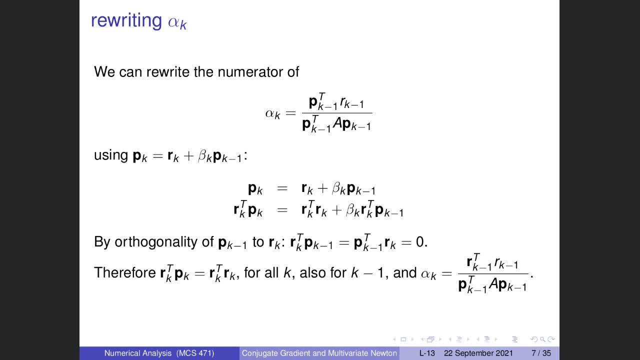 Residual Of The Vector. Why Do We expression? but if you think about the first exercise, it may actually also save us some time, because note that this is actually what you use. this inner product is what you use in the. 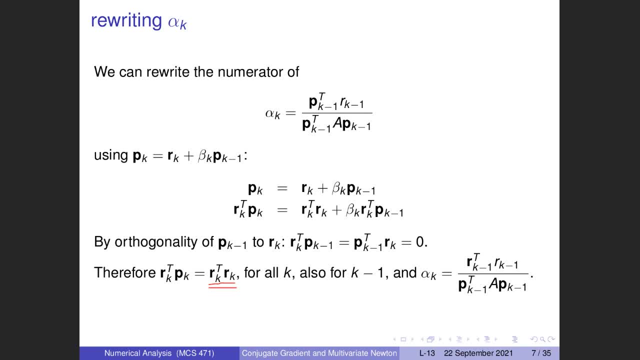 two norm. So in the first exercise you had to compute a two norm, a two norm of a vector, and for the two norm actually you get the inner product of the vector with itself, And here you can see that you can recycle that So we can rewrite the numerator using the expression for. 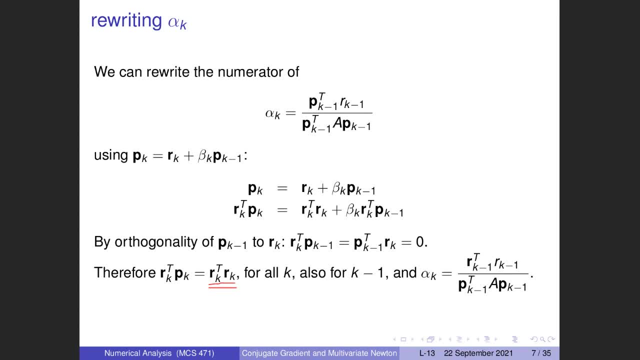 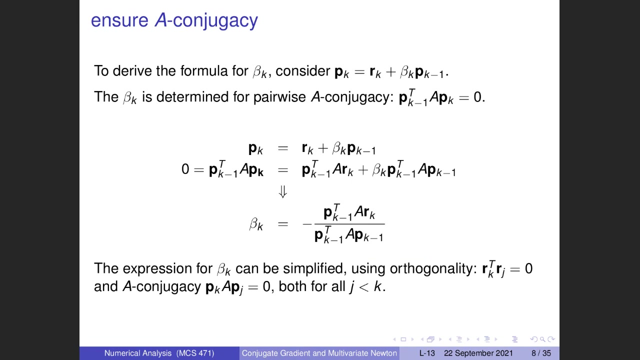 the update of the direction vector. So, and we then also use the orthogonality to rewrite the relation. So we actually do have that, the, because this is zero. we actually also have the orthogonality property. Okay, so this gives us a neat expression for alpha k. Now where does the beta k comes in? And this: 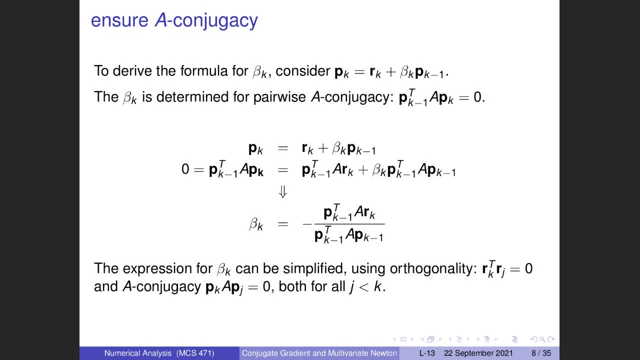 was also to explain the name of the conjugate gradient. So we had this more complicated norm where we use the A matrix. We actually have now that the directions, the gradients are actually conjugated to each other. they are related. So奦o, conjugating is a little bit more fancy word for relations. 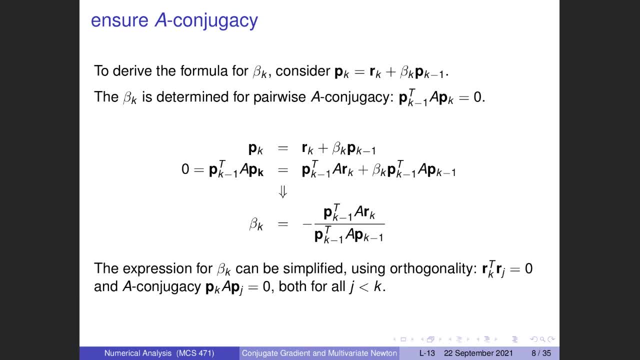 They are related to each other by this matrix a And by actually using, by enforcing distributed wwwdetост window. we shouldn't be hoping it will come into that. Let's, Kimberly, continue to questions by looking at your questions wherever these questions arise. He's joking, but start to think this over a little bit. If you'll hesitate a little bit, All right. of course you might want to see how. Okay, so can you go back to the WhereNumbervas University described thattalk that we made earlier today. 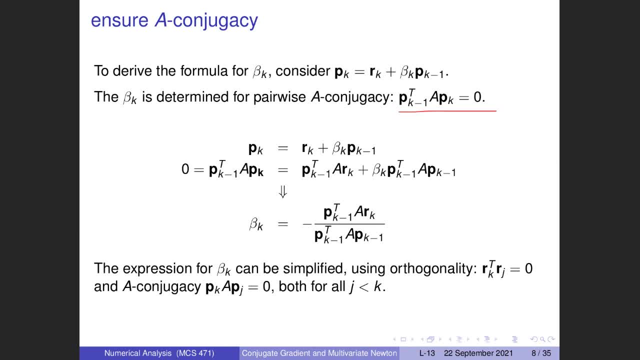 Yes, that's right. Okay, All right, thank youσι Wars. enforcing this new condition of the conjugacy that will lead us to an expression for the beta. so the beta that then here, still has this in this matrix vector product in its numerator. 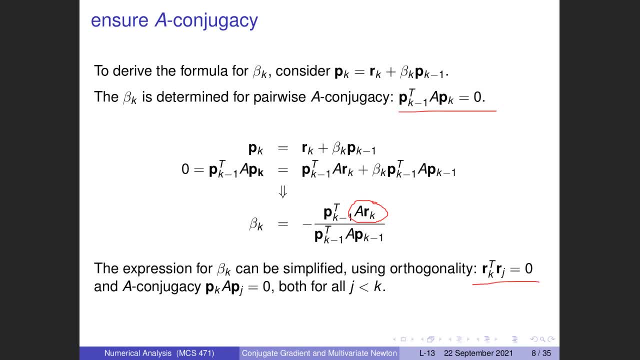 so this can still be simplified by using again the orthogonality and that gives then the expression for beta k that was used in the mathematical description of the algorithm. so in the little slides that i have used here so far i've tried to explain the algorithm and kind of in a backwards manner. 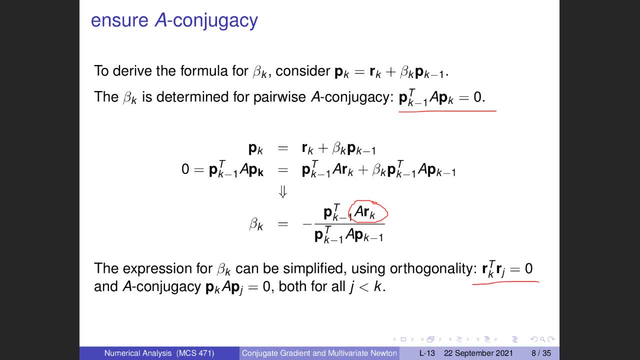 uh, so we started with the formulation of the algorithm and then we're going to derive essentially the algorithm, and so there are some key parts in this. the algorithm will actually ensure that the residuals are orthogonal to the update vectors. that gives them the formula for the alphas. 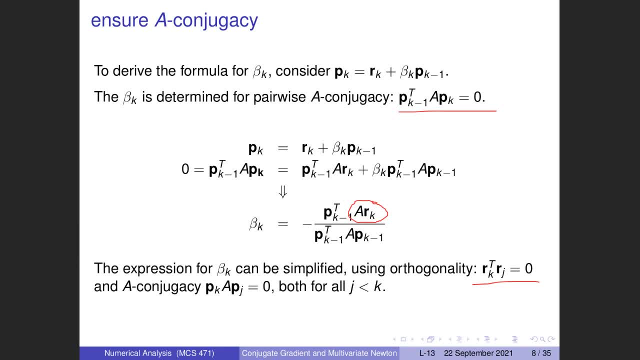 for the step length, and the other condition is that we do have this pairwise conjugacy on the uh direction vectors. you also actually now recognize the condition that we used to minimize. so actually we were minimizing the norm of e- e and that was e transpose times a times e. so that's the square of this uh special. 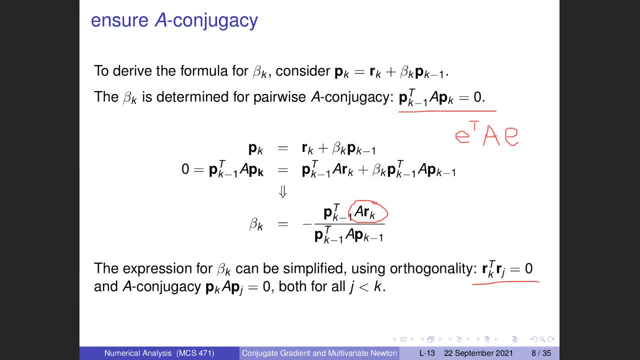 norm and you see that the norm of e, e and that was e, transpose times a times e. so that's the square of this, uh, special norm, and you see that this is what we want to minimize and we actually also want that. if you, why do we actually do this? well, at the 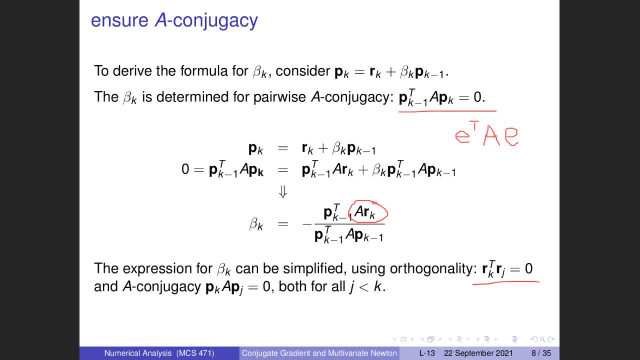 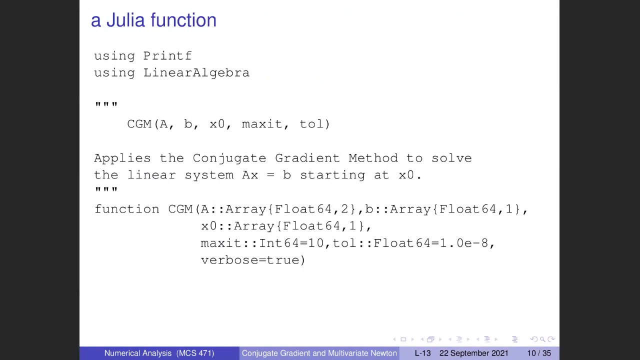 minimum. everything is actually zero. so the directions in which we have to go. there is no other direction to go. we are already at the minimum. so that's why we actually enforce, uh, this condition of directions. all right, um, we define our algorithms by julia functions in this course. 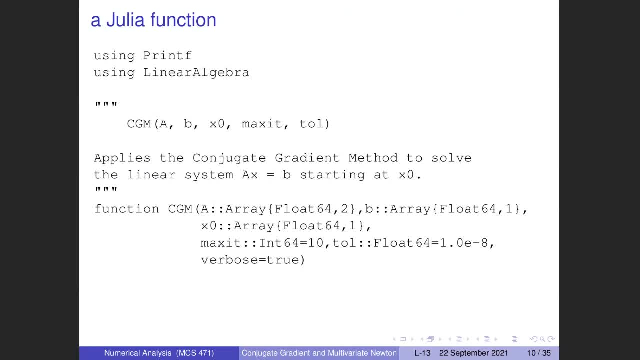 so we will have a conjugate gradient method which has six arguments. so here my documentation: string leaves off actually the default verbose option, so there is an extra verbose option, so it's an iterative method. uh, in addition to providing the coefficient matrix and the right hand side vector, 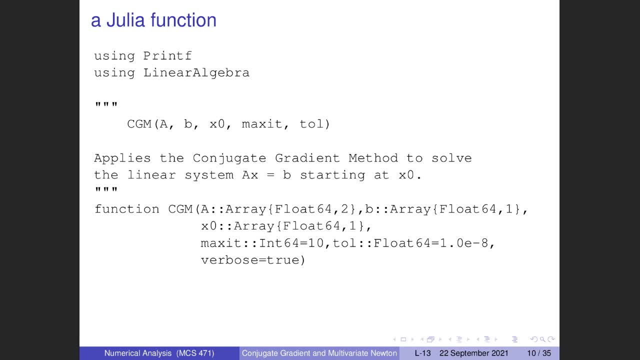 the user must provide a start solution. uh start vector. if you don't know anything, give zero. that is as good a start factor as any. so we have default uh tolerances. uh, default tolerance of 10 to the power minus 8 and 10 iterations. that's because 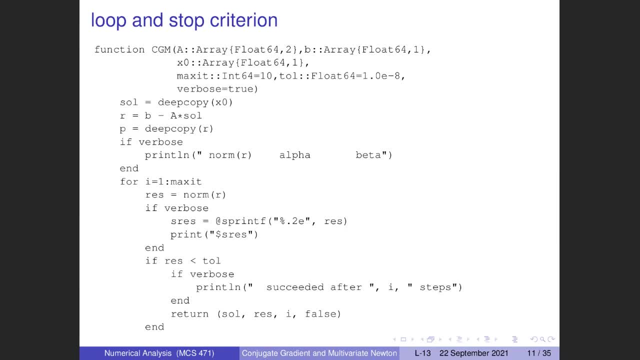 i tested this on very small examples. all right then. um, we start out uh, with the initialization of the x, which is now actually called sol. we have our residual and then our uh direction p, which will be initialized to the residual. so this is no longer a mathematical. 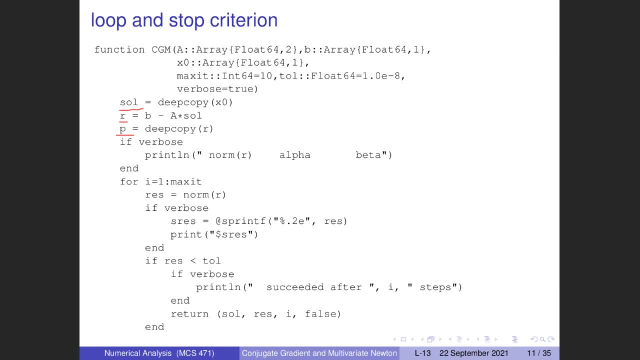 algorithm, we will have only one solution, only one residual vector and only one direction vector. So typically we have our stop criterion at the end, But here you see that everything is actually now at the beginning. So we have our stop criterion on the number of iterations and we have then stop criterion on the residuals, which is the norm of the residual vector. 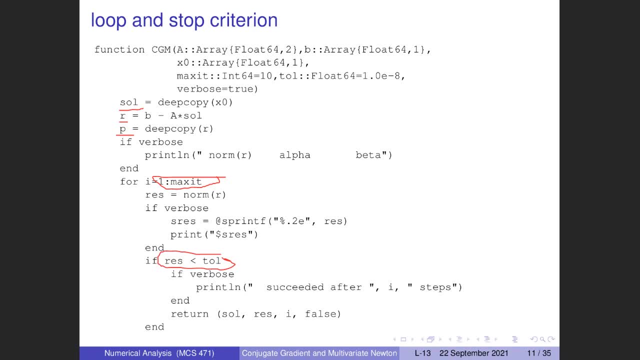 So the algorithm starts out like this: now, and then we have the printing, So we actually will print out the values for the coefficients alpha and beta, because they actually should go to zero. So that's actually important. It's a very important property that I forgot to point out. 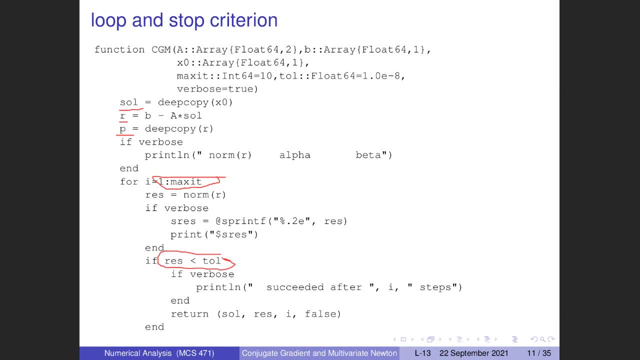 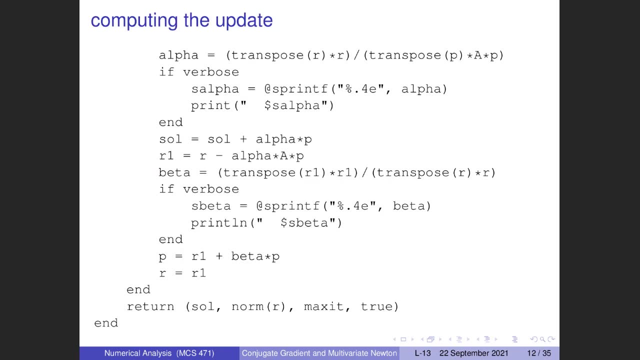 The alpha and the beta have both in their numerator the residuals. All right, the algorithm. So here it is actually. So here you see the numerator for the alpha, You also see the numerator for the beta, So you see that They both have the norm of the residual sitting in there. 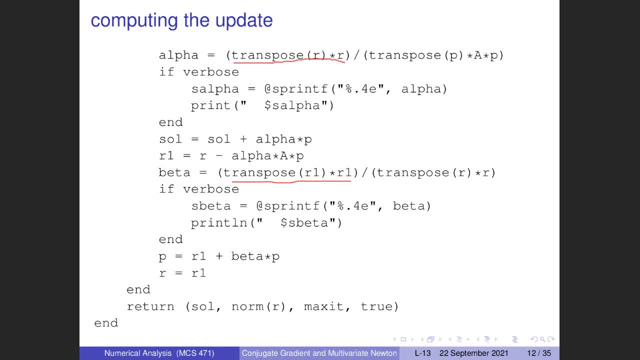 So actually all these numbers are the alpha and the beta. They should actually all go to zero if we have a converting process. So in a way you could interpret this conjugate gradient method as kind of an elaborate way to check in three different ways. 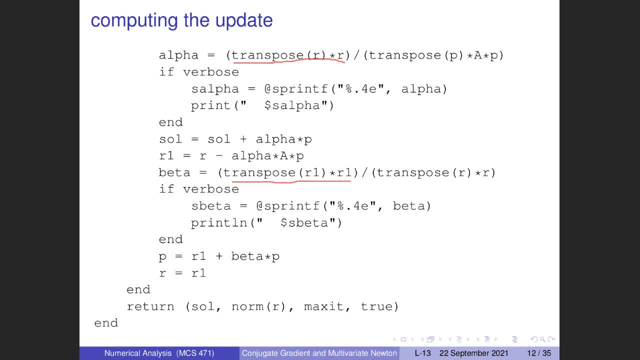 Actually are we actually there yet? So It's very, very small. If your step size get very small, then actually you are already very close to the. So I'm sorry, I'm sorry, Sorry, Sorry, Sorry, Sorry. 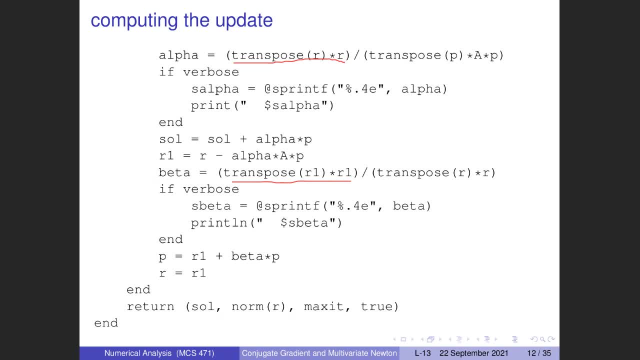 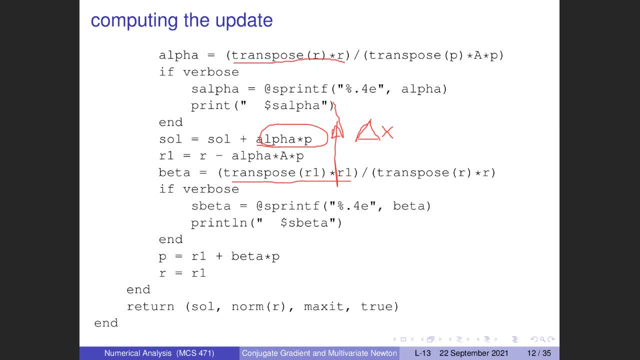 Anyway the next. So I'm sorry, My internet was a bit Unreliable So let me redraw it again. So the Delta ex Is actually here, The alpha times Speed, Then actually you can see We have only 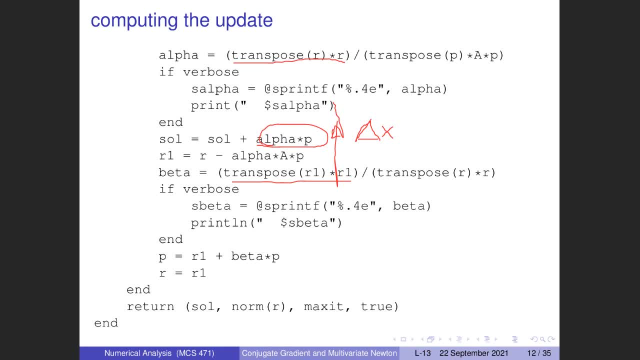 The size of the update. There is the update of the solution and then there is the update of the direction, That is for which the beta coefficient is being used. So this is a very simple algorithm, Simple enough to work on very high dimensional problems: Many equations, many variables. 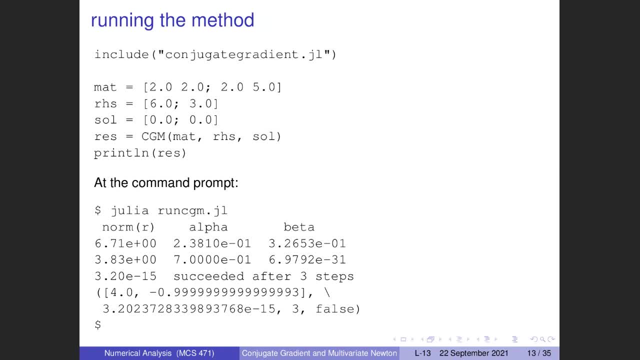 But we do this here on very small systems. Here I have a very small example that fits in one slide. So execute the test At the command prompt And you see that we actually are converging extremely fast. So in actually a couple of steps, in two steps, we actually have success. 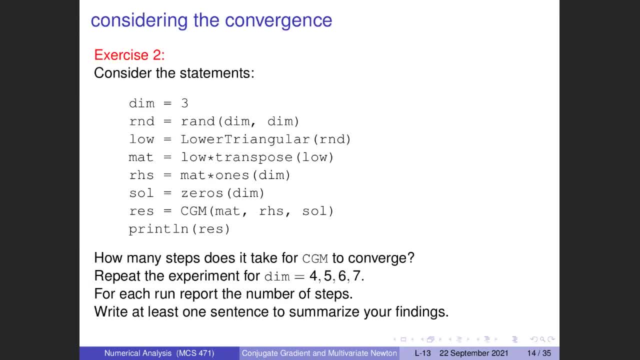 All right, Very good. Here is another exercise. So this is an exercise, which still is for a small dynamic. So you execute the statement. So we will look at increasing dimensions. So you execute these statements. Note the way how the matrices are formulated. 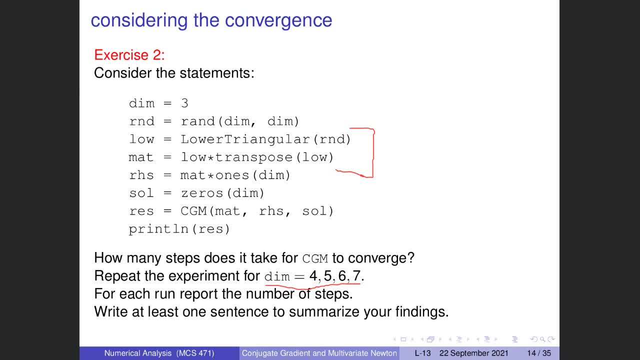 So this is an optimization problem. We are looking, we are applying a variation of the steepest descent method, And when will this work? well, When our form one, our quadratic form that we will minimize, will actually work on a positive, definite matrix. 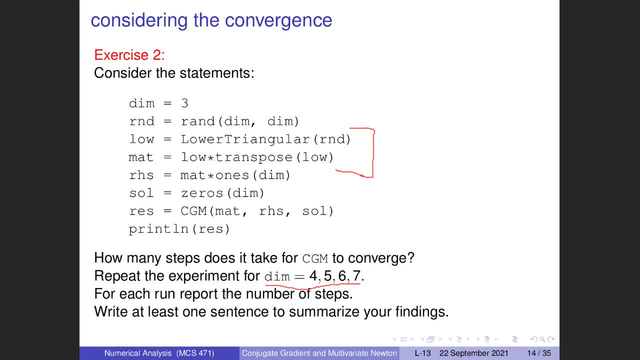 so it has the same convergence uh conditions as we assumed for the koleski factorization. so you can actually consider we have seen the methods of jacobi and the relaxations of gal side l, which were kind of the iterative uh variations to the direct lu factorization. we have the direct koleski factorization for which is a direct 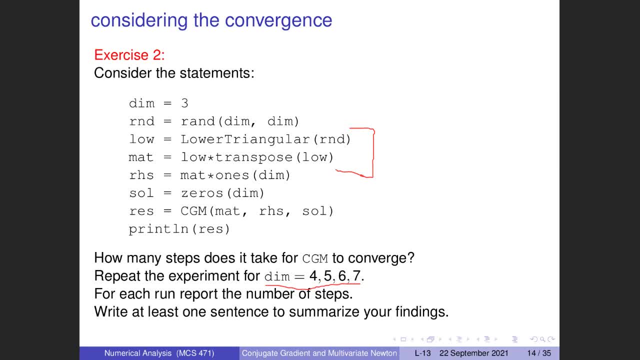 method, not an iterative method, which works well for positive definite matrices. here we have the positive uh definite version for large problems. now here i'm generating my positive dimensional matrices, my positive definite matrices, in the very straightforward way. by the end of the last lecture we saw that that was actually not such a good idea. 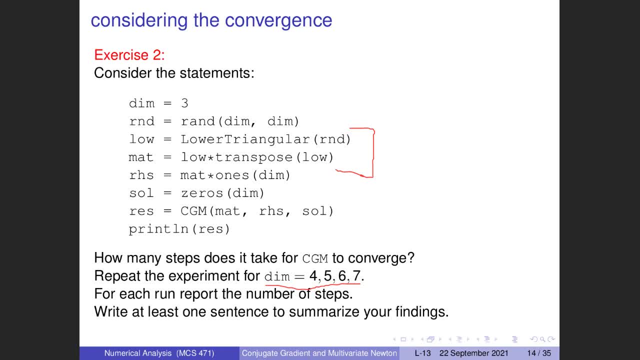 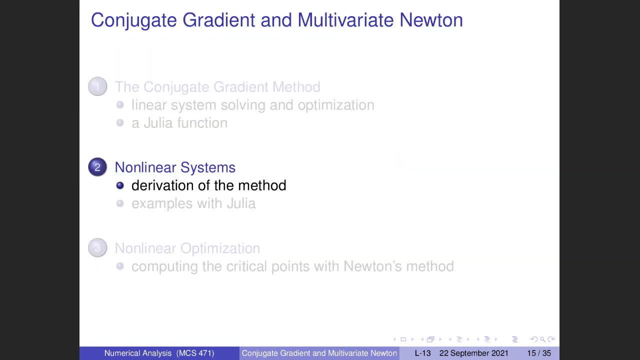 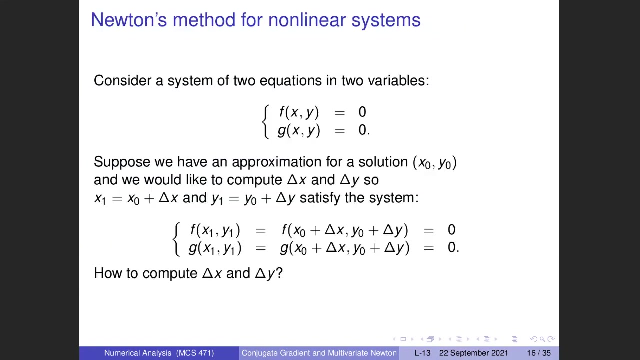 so in a way, this will. this exercise is mainly to investigate the convergence, so see how it converges, is should happen, because these are still very nice positive definite matrices. all right, we've seen gradients, so let's now move on the jacobians. so we've covered newton's methods to solve linear f, to solve non-linear equations. let's now look at 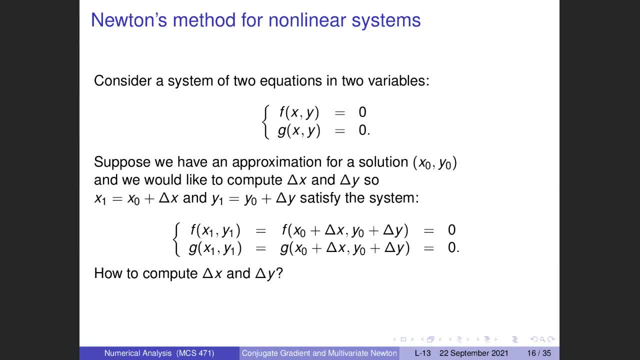 the more detailed general case and let's look at a system of two equations in two variables and in an iterative method. we like to compute updates so that we are closer to the exact solution. so the system is given to us with variables x and y. we have somewhere. 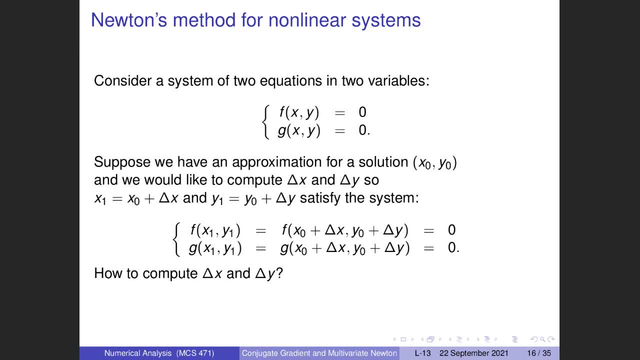 a first approximation for the solution. so x naught, y naught. first of all we check whether it it makes it zero or not, but most likely, otherwise we wouldn't really have anything to do. so we will compute a delta x and a delta y so that we will get close. so we 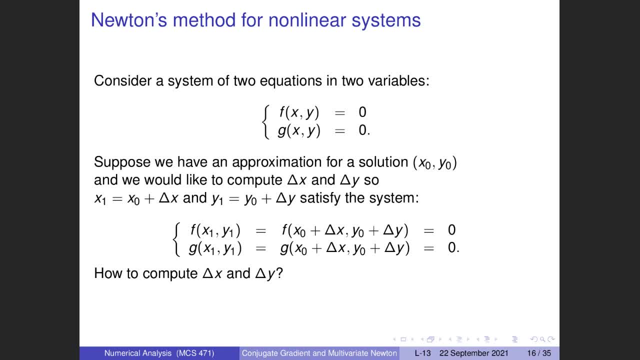 actually reformulate the original problem into a positive derivative and you can see that we can compute the question of what is the interesting thing with that. so we can say that we go to the into a problem where the unknowns are actually now the delta x and the delta y. 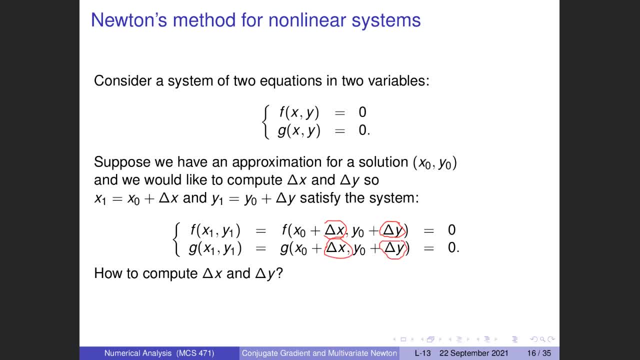 So we have two equations in two unknowns. Why is this a simple problem? Well, we actually hope that the x0, y0 is already close. Then, actually, we are looking for small numbers: delta x and delta y. So now, how do we compute this? 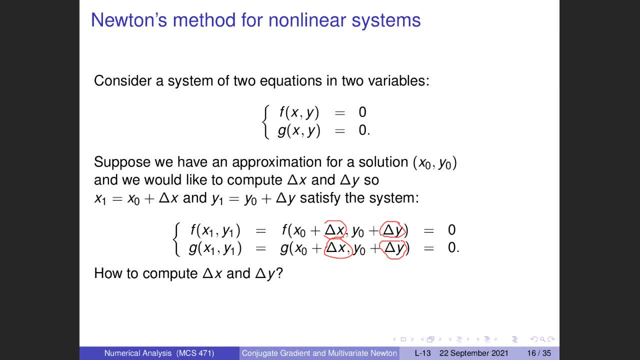 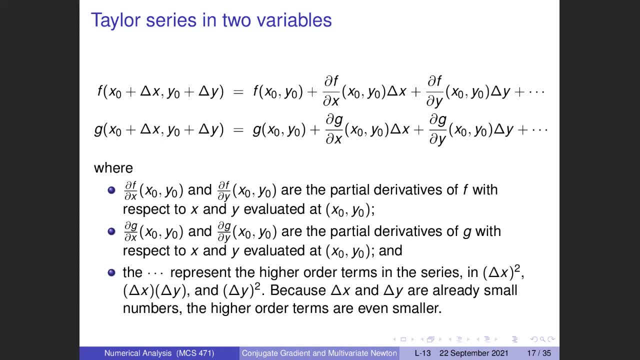 Well, the delta x and the delta y are small. That means that we can apply Taylor series. So Taylor series, we have seen, were an alternative way to derive Newton's method. Newton's method is also called the tangent method. In a way we could also give here a geometrical interpretation. 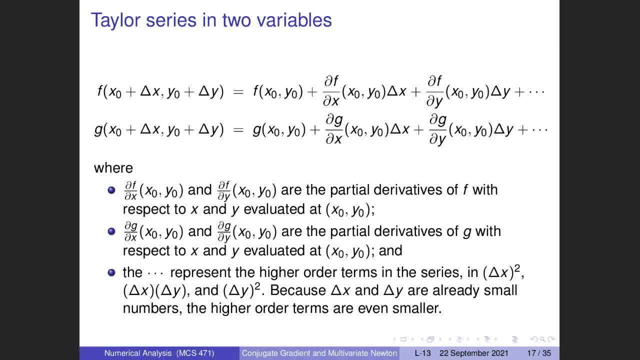 by using the tangent at the intersection of the two tangent planes. So in tree space we have two tangent planes and two planes intersect in general in a line. So the two tangent planes will give us the tangent line And you could interpret also the Newton's method geometrically. 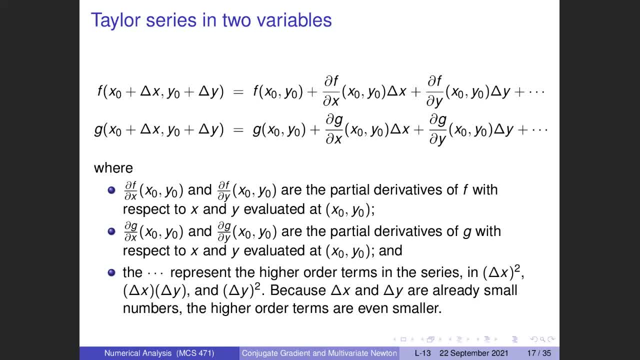 So it would be a very good exercise- I haven't done this yet- To actually to actually give that geometric interpretation, But we will work with Taylor series in several variables. So now we need the partial derivatives which we remember from calculus. 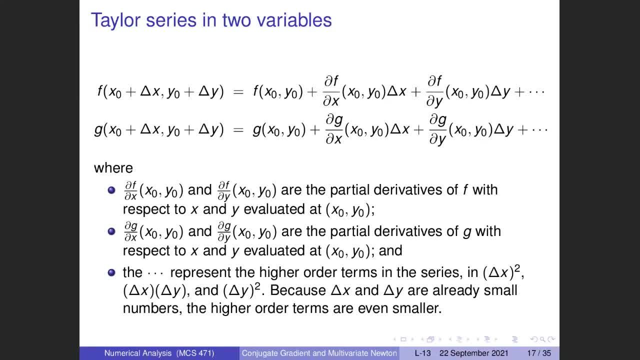 You take the derivative with respect to one variable, treating all the other variables as constants. So we ignore the higher order terms. So the dot here contain the delta x square and the delta x times delta y and the delta y square, Because all the delta x's and delta y's are actually small. 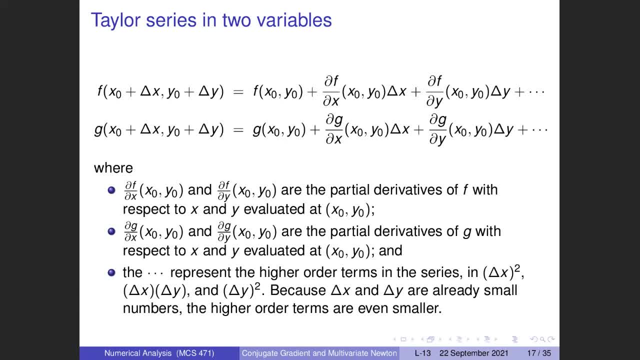 we can do that, So we actually will truncate those. So forget about the dot dot dot. And what is the punchline now? This is a linear system, So this is why Taylor series are so very powerful Locally. everything is reduced to a linear system. 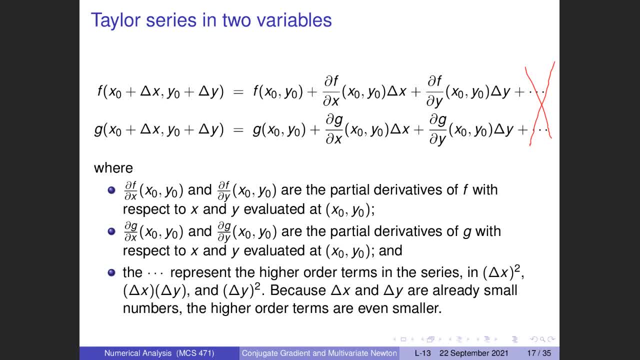 It's not obvious from here. So this looks like a problem with a lot of letters And it's important to realize that delta x and delta y are actually the two variables And we will formulate this now as a linear system In the future. 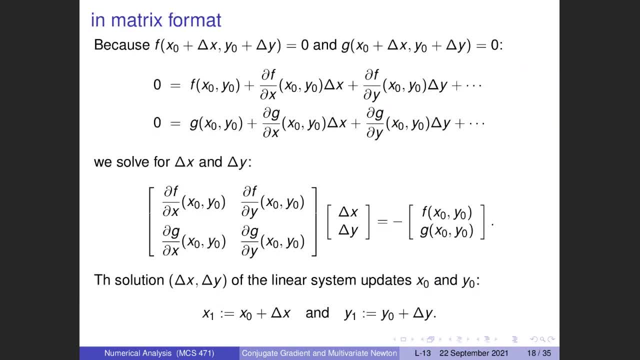 We will use the proper notation using matrices. So I've copied, still with the dot dot dot of what I had in the previous slides. So what do we know? Well, we know the x-naught and the y-naught And what we actually did. as I said, we evaluated. 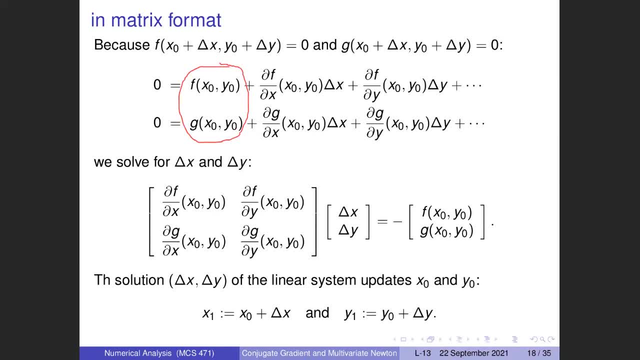 So we evaluated the x-naught at f, x-naught, y-naught at f and at g And that will actually make the right hand side. So it's not zero. So it has here a negative sign Because we want to solve this equation for delta x, delta y. 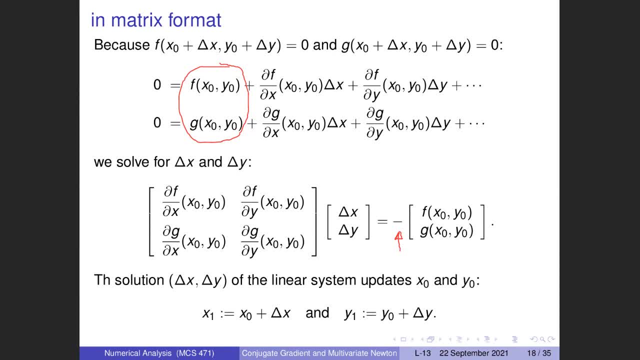 So then, what we also know are actually the values of all the partial derivatives, And that will be the coefficients in our matrix. So what we don't know are the delta x and the delta y, And that will make our update vector, And actually we solve one linear system. 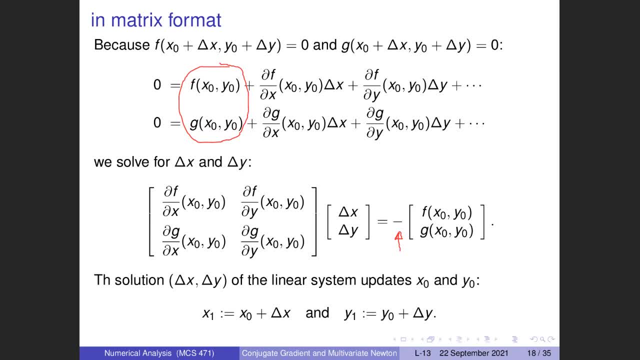 And the linear system will actually give us the correction terms to the current solution. The magnitude of delta x and delta y of that vector will actually give us an estimate for the forward error. So in a way, if you look at this formulation a little bit carefully, 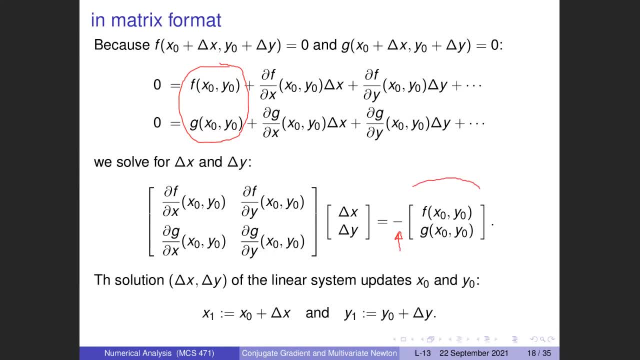 So at the right hand side we have the backward error or the residual At the left. here, what we want to compute, we actually have the forward error. So you can also see Newton's method as a method to try to connect forward error with backward error. 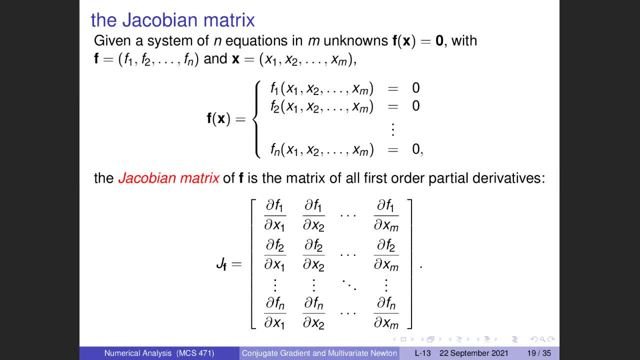 All right. In general we have a system of n equations and n unknowns. So for this lecture n is still equal to m, And later in this course we will see that n can typically be more than m. But in great generality we have the matrix of all first order partial derivatives. 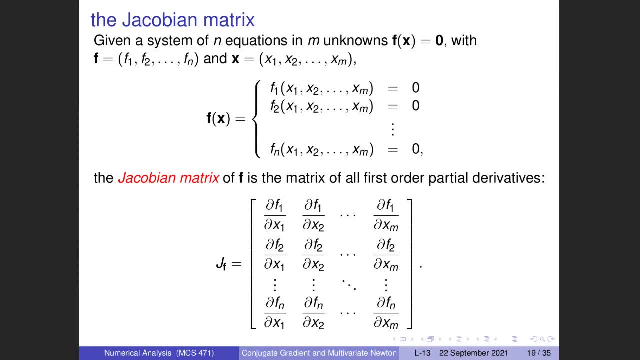 And that is called the Jacobian matrix, And that's a matrix, a genuine. So here it is formulated as a matrix of nonlinear functions. So you can see this also as a function of a vector that returns a matrix. So for any value of the variables, the x variables, you get a matrix back. 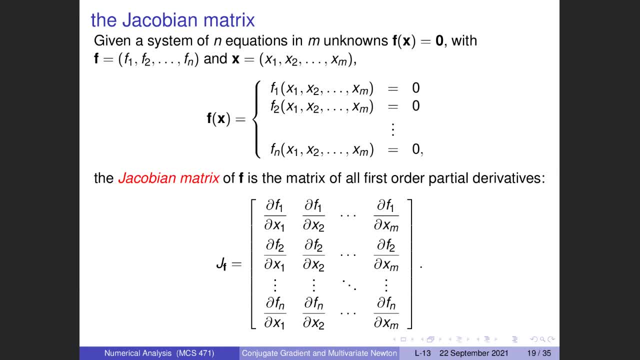 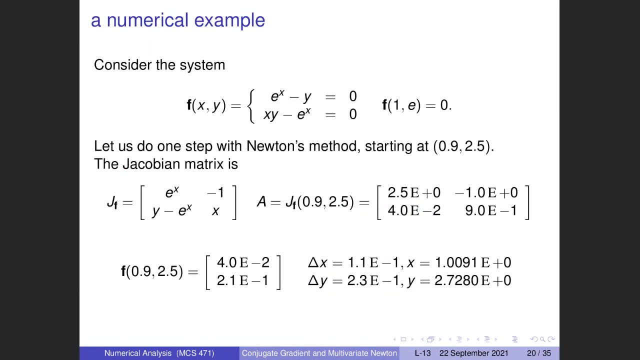 So this gives us the coefficient. So you see, the indexing first row deals with the first equation. So the second column here deals with the second variable. So there is a very natural way to order these elements in the Jacobian matrix. Here is an example, a numerical example. 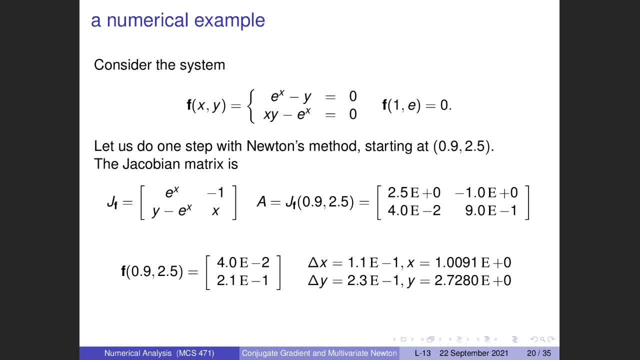 So we have a nonlinear system, but still a nonlinear system where we actually know the exact solution. So we compute the Jacobian matrix And then we compute the updates by solving a linear system. So this is a numerical example dating from the time of the scientific calculator. 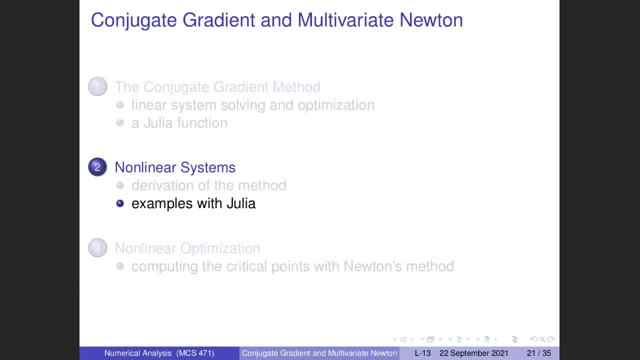 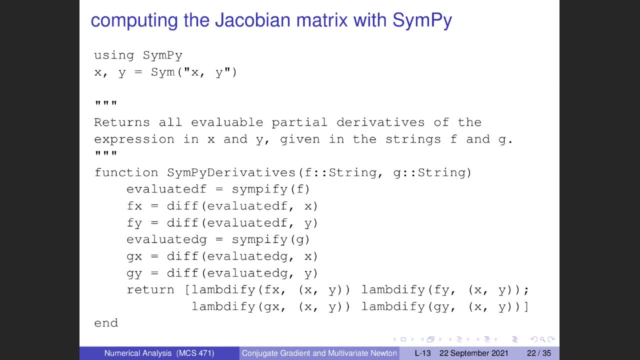 All right. So we are going to implement this in Julia using SymPy, So generalizing here to two variables. So it would be an interesting exercise- but that's an exercise in symbolic computation- to make this work for any number of equations and any number of variables. 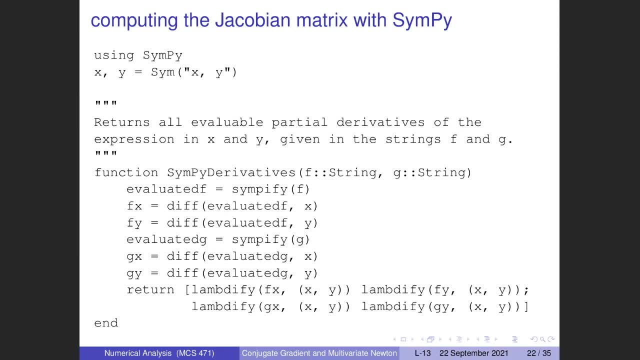 But we do this here in two variables And that's just generalizing the functions that we have covered when we first introduced the Newton's method. So our expressions are given as strings, parsed into SymPy expressions, with SymPy using the global definition. So the SymPy works within the global context where the x and y are variables that are occurring in the strings. 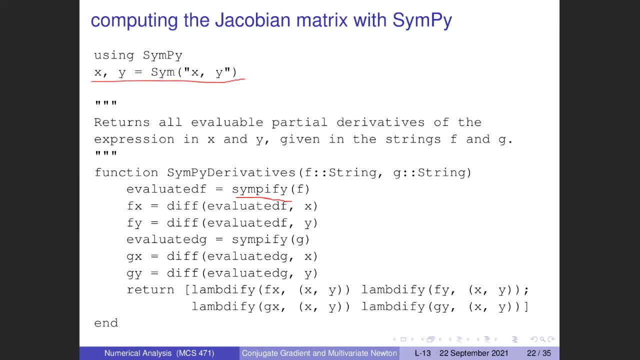 Once they are simple expressions, we can evaluate and, more importantly, differentiate them symbolically And we lumbify. The lumbify actually will return functions. So we have the expressions for the derivatives and they are turned into functions. So we will actually have a matrix of functions that we can evaluate. 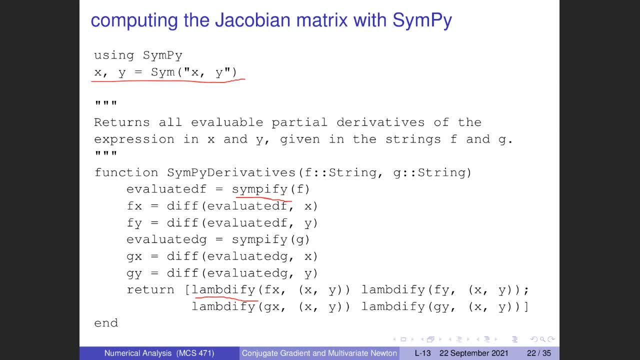 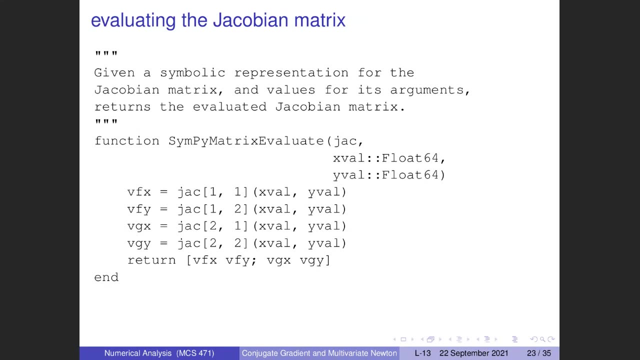 So this is what is essentially very simple function is doing: It takes strings on input and it returns a function to evaluate the Jacobian matrix. Here you see how this then actually happens: The lumbified expressions can be evaluated numerically, So, and we return a matrix. So this is here. Everything is happening here with the 64 bit representation, with the 64 bit floating port numbers. 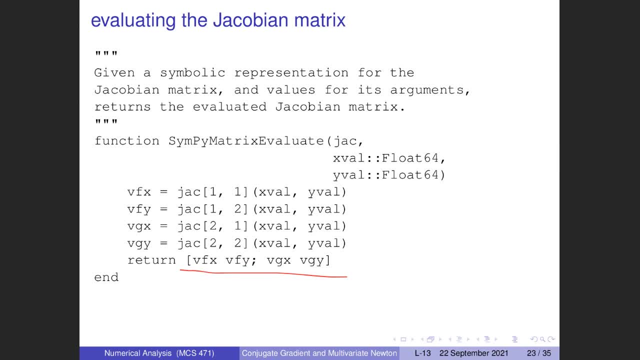 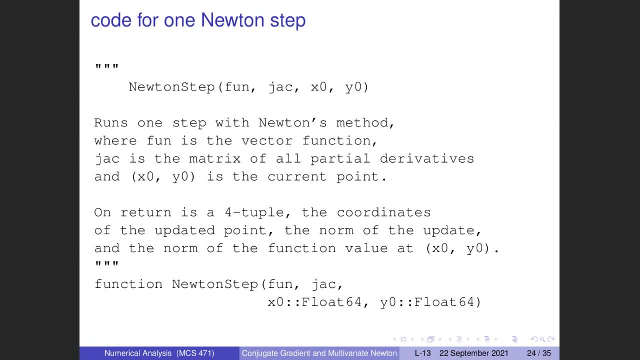 All right. So these are the auxiliaries, And now we can define Newton step one, Newton step in great generality. So what we are having on input are the vector function that evaluates the nonlinear function, And then we also have the linear function. 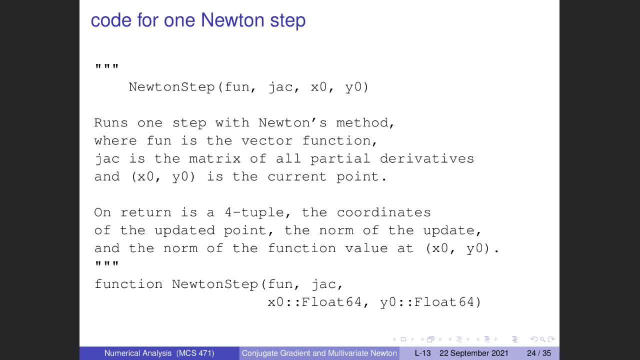 And then we have the Jacobian function And we start with the current point. So this is extracting the body of the loop in an iterative method by a step function. So in a way sometimes it's confusing to think about the entire iterative method. 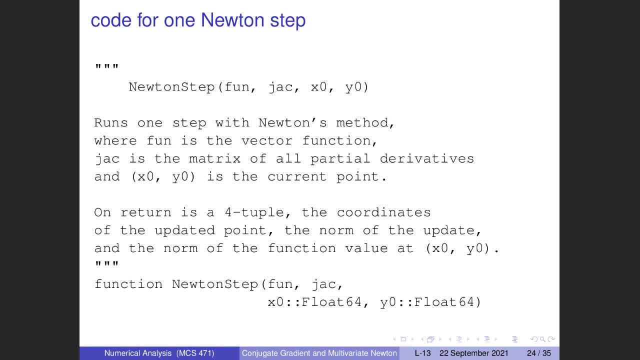 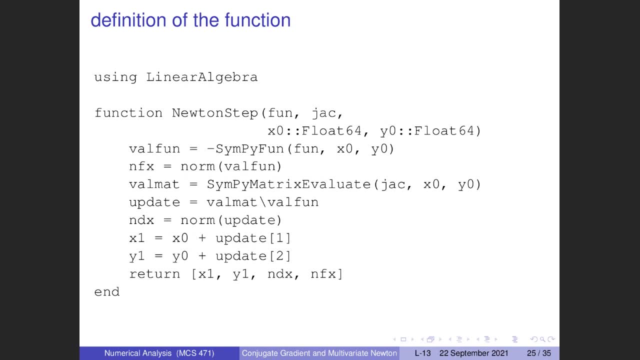 Well, first isolate the function that computes the next point in the iterative method. That's what this Newton step is doing. So, and here comes the linear algebra. and the linear algebra is entirely encapsulated by the backslash operator. So we use the built in linear algebra module, built in with Julia, and we compute the update by the solving of a linear system. 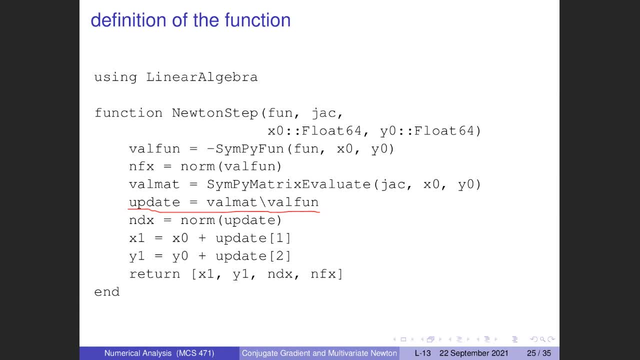 Then what we return is the next two values plus the norm. So here we have the estimate for the forward error and the estimate for the backward error. So we in for well conditioned problems. if everything runs well, they are of the same magnitude. 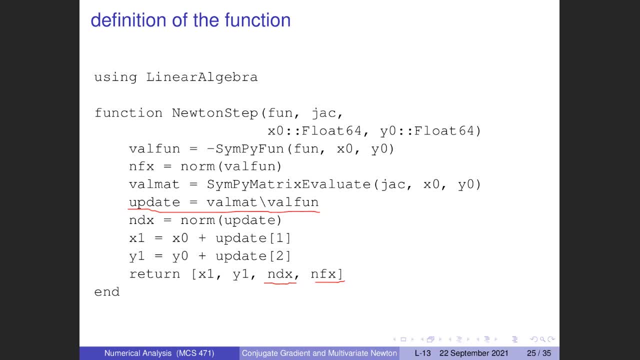 When the backward error is small, also the forward error is small. So we have the next point in the iterative method and two quality and two floating point numbers that will tell the quality of the approximation, The estimate for the forward error. So this was here, the delta x. 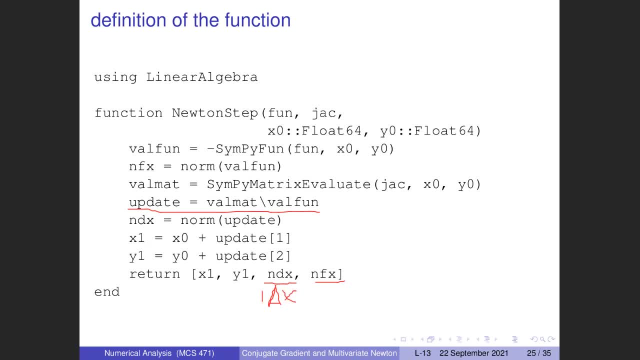 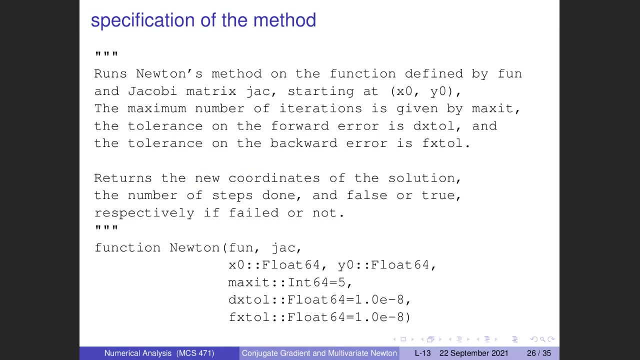 It's norm. And we have then the norm of the residual. So the residual was b minus a times x and linear out Here it is the residual which is the norm of the function evaluation. All right, So then we have the iterative method, where we will have again quadratic convergence. 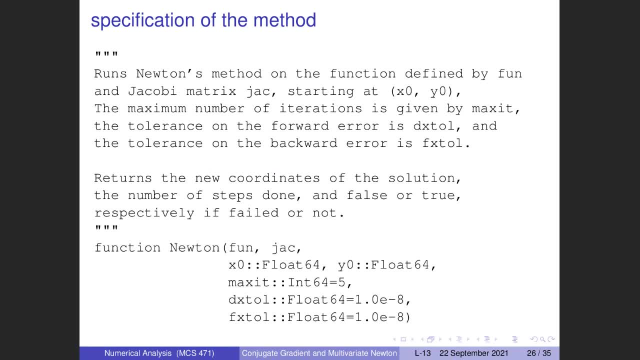 So we do not allow that many iterations. If we require a 10 to the power of minus eight, we only allow five iterations because we expect quadratic convergence. So the default tolerances are set up with that in mind. Of course we will see that this is not always satisfied. 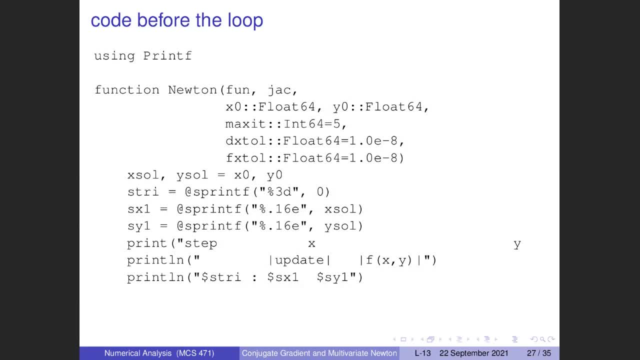 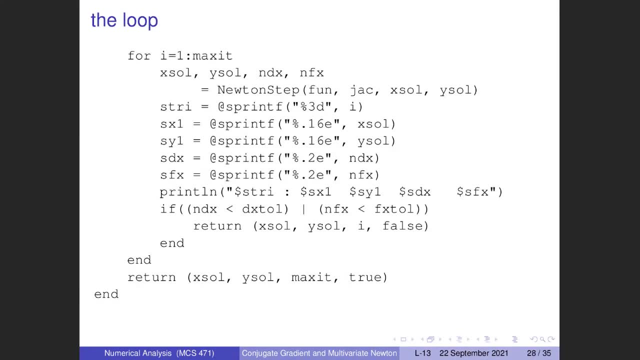 Then the definition Of the Newton method is actually an encapsulation of the Newton step. So where we do the updates, So this encapsulation happens here. And the advantage of the encapsulation is that when we write the Newton we can focus on the layout. 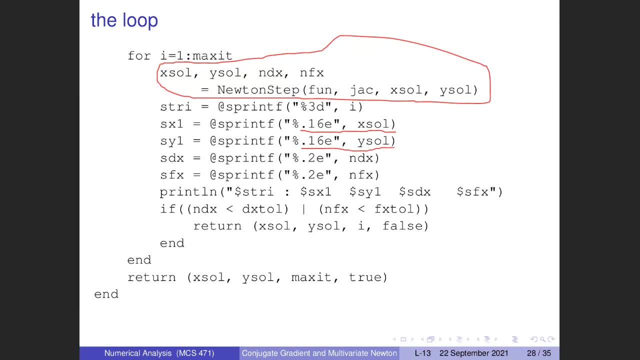 So the solutions are: The solutions are printed out in their full precision of 16 decimal places: The estimates for the forward and the backward. These two norms are given only with two decimal places And the method may fail, So that happens here. 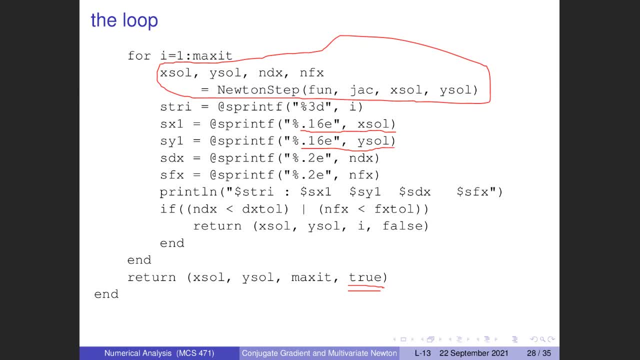 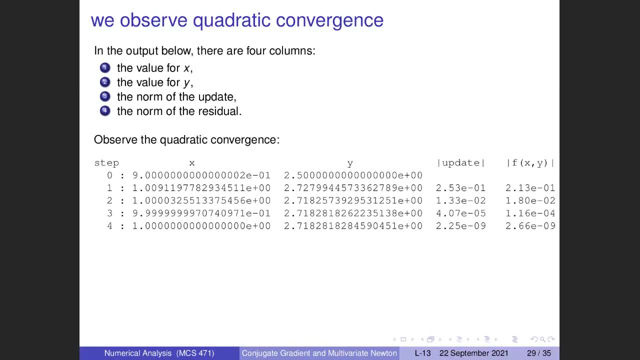 We have failure. Fail Last variable is true When we have exhausted the allowed number of iterations And have not reached the tolerances. Here is a very nice example. I think I took again the example with the E value So you may recognize we have the transcendental constant E again. 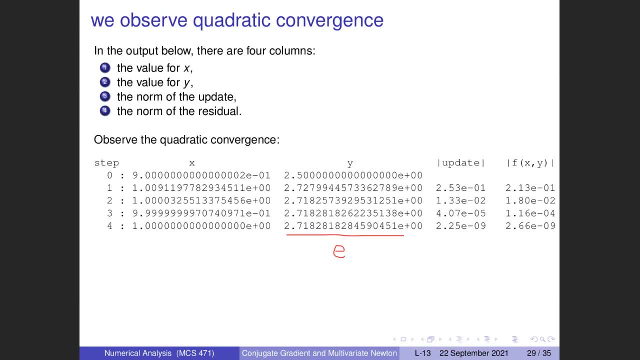 To its fullest precision, most likely Because the update, last update, is actually less than 10 to the power minus eight. So let me just erase that. And, most importantly, you observe the quadratic convergence. There is also always a pleasure to see this. 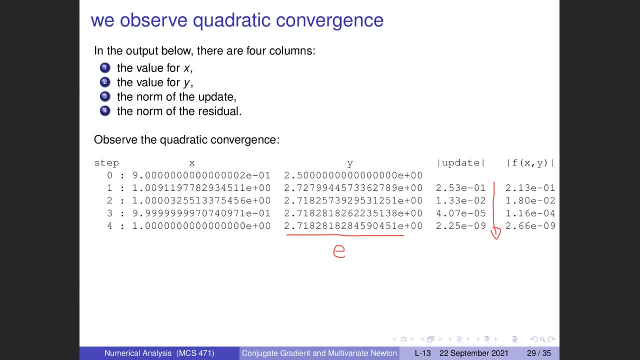 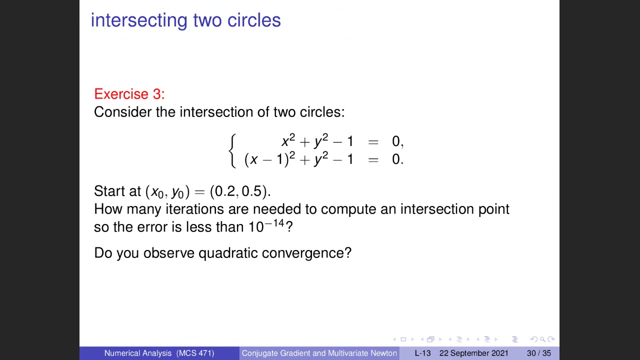 You see that the exponent actually doubles in every step, Or almost doubles, Doubles a little bit more, A bit less, And the exponent is negative. So doubling exponent that is negative is an indication of quadratic convergence. Here is a very simple example, but still intersecting two circles, and you can have some applications. 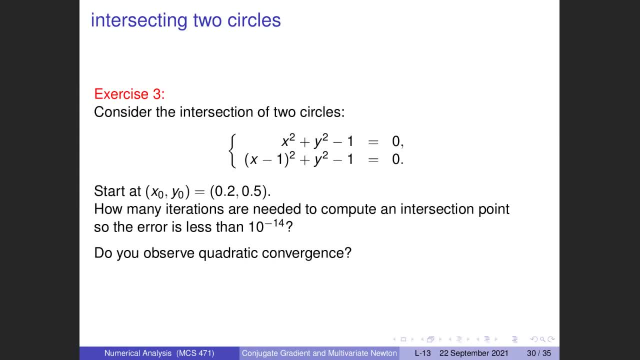 So run the posted code and run it for the two equations, f and g, to the equations for the circle. The question is: do you observe quadratic convergence? The answer will be yes And in essence this is a sanity check on how accurate, on how you have adapted and copied into your Jupyter Notebook. 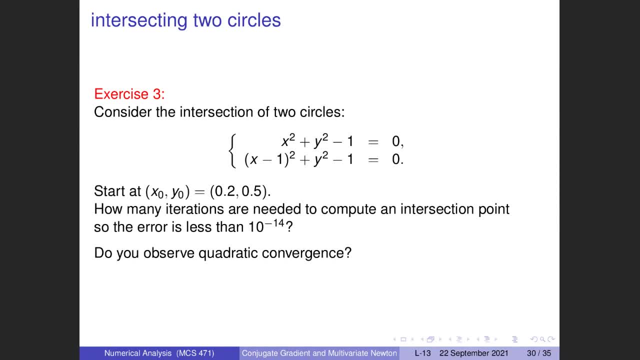 the definitions for all the pieces that are posted as a Julia program. So again, the answer is yes, But show all your work. One can also say that suppose that you would know that you have here one decimal places correct. How many iterations are necessary? 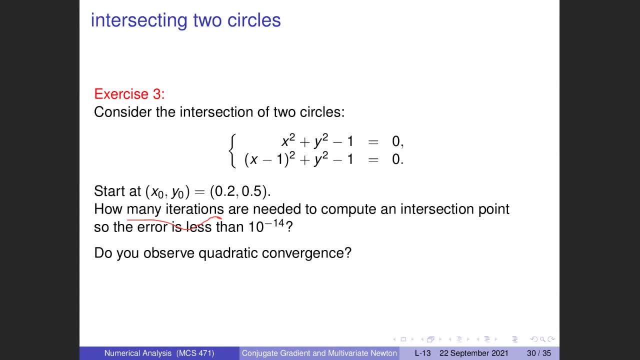 You can actually calculate that without or estimate that without doing any actual computations. So you go from minus one minus two minus four, minus eight, minus seven, minus eight Minus 16.. Five steps: Minus one minus two, minus four, minus eight minus 16.. 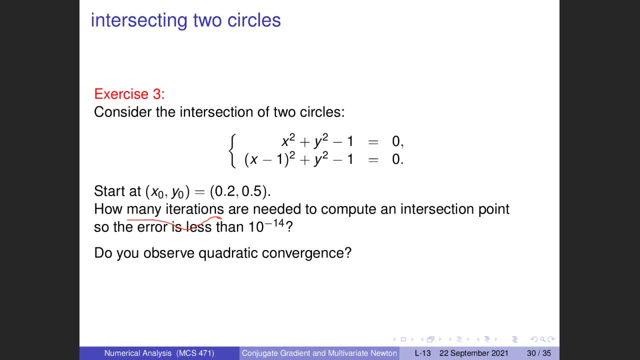 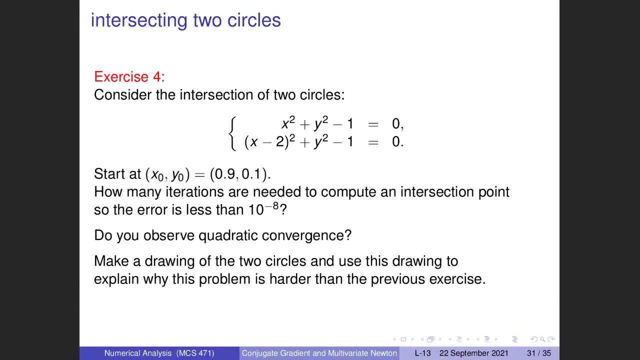 So this is why this is justification for the default of five. Assuming that you start with one decimal places accuracy in your start point. The next equation, the next problem, is a lot harder. So we have circles. So I should actually made a plot. 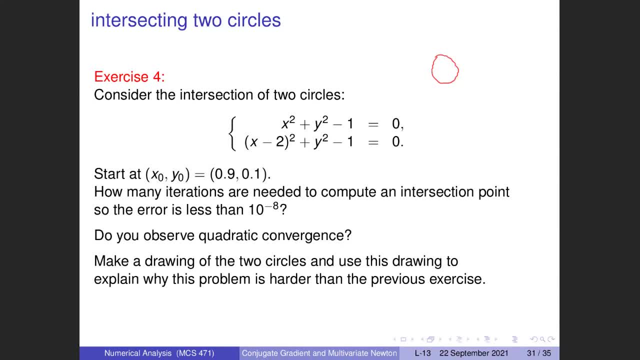 So you have one unit circle centered at the origin, And then you see that the odd circle is centered at two and also has radius one. So these are two touching circles, And the answer will actually here be no. You will not observe quadratic convergence. 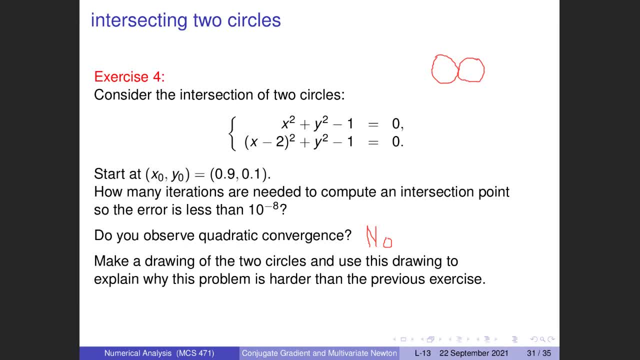 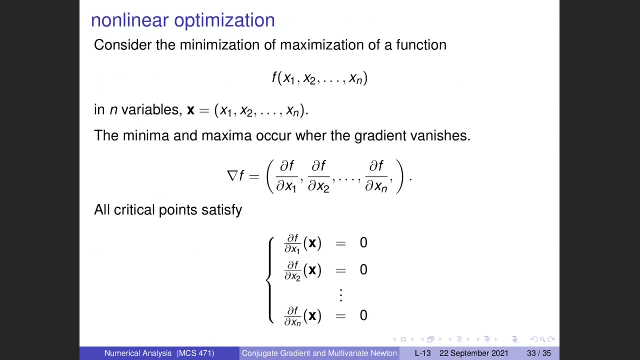 So the drawing actually explains why This is a harder problem. If you run this, you will see that you may still observe linear convergence. Now we will not go into this. So analyzing multiple roots in multiple dimensions is a lot harder than we did for one equation. 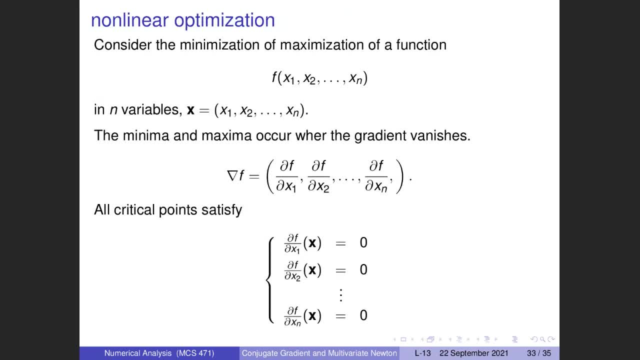 Last slide, almost. So where do the Hessians then come in? Well, if you consider the application of Newton's method to minimize or maximize a function, then you will look at the linear system or the nonlinear system that is defined by the gradient. 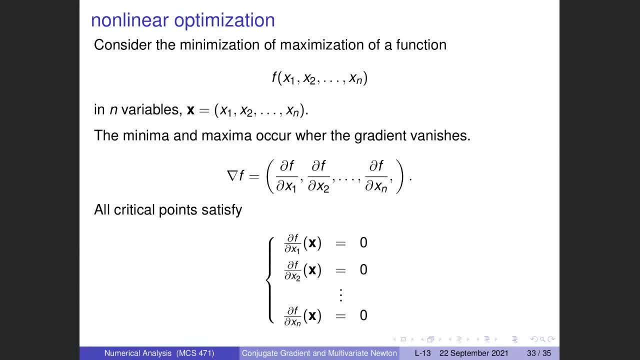 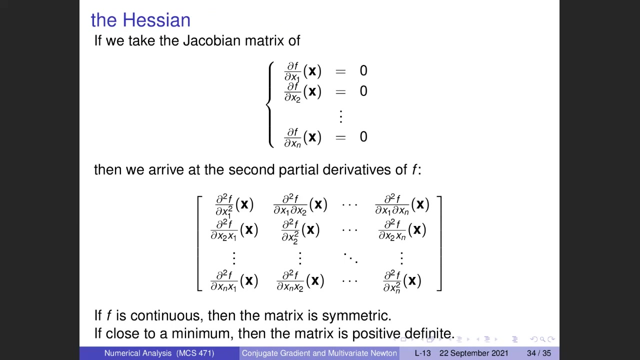 So because the gradients, actually the solutions of the gradient system, now actually satisfy the critical points, So the candidate minima or maxima. You can also have samples, as you remember, from multivariate calculus, So a nonlinear system to which we will apply Newton's method. 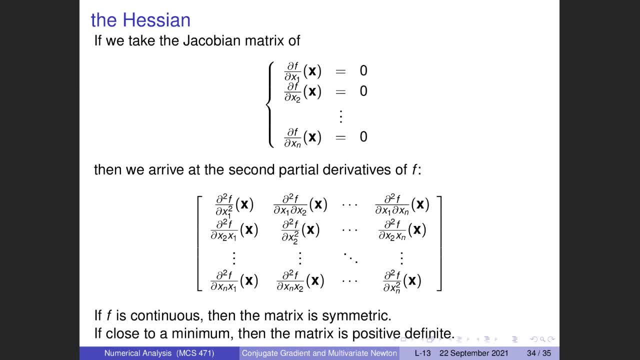 And here you see, the point of this slide is actually to indicate that where do these symmetric, positive, definite matrices come in? Well, they come in from taking the Hessians of the Forms that we try to minimize. So here, if you take the matrix of second partial derivatives, in a way, you take the Jacobian of this. 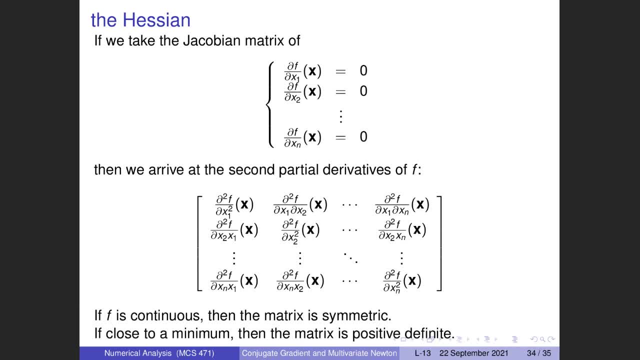 then you see that we have a symmetric matrix. if the function is continuous And if you are close to a minimum, so your function doesn't need to be entirely special. But if you are close to a minimum, so your function doesn't need to be entirely special. 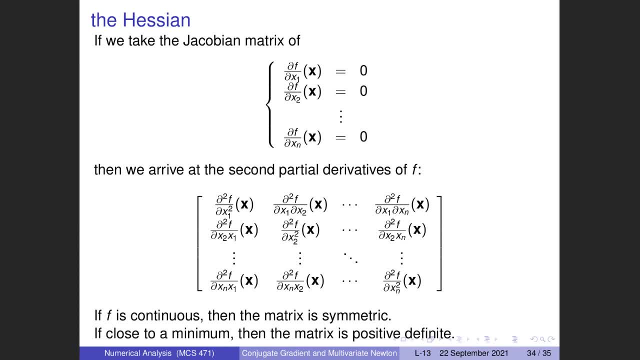 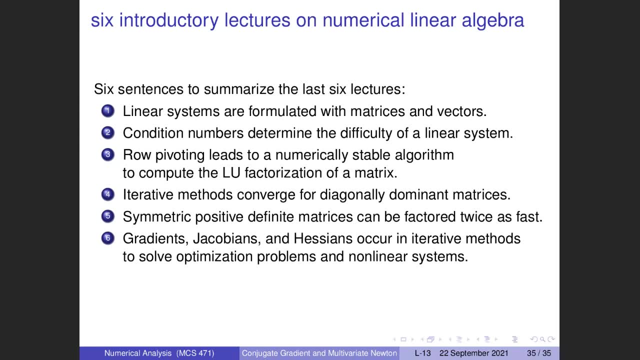 But if you are closer to a minimum than your matrix will be positive. definite: All right, Six lectures. we have covered. It's all linear algebra. There are six sentences that summarize the last six lectures. So we use matrix and vector locations. Condition numbers are very important. 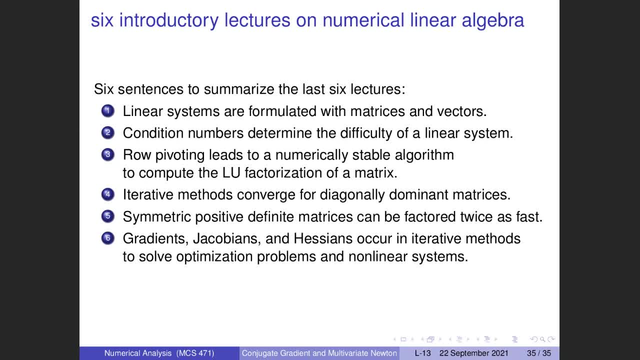 To determine how hard it is to solve linear systems in this. So if the condition number is too large we can't really do anything anymore. But in this course we care about numerically stable algorithms to compute Here. as we have seen in LU factorization iterative methods converge for diagonally dominant matrices.